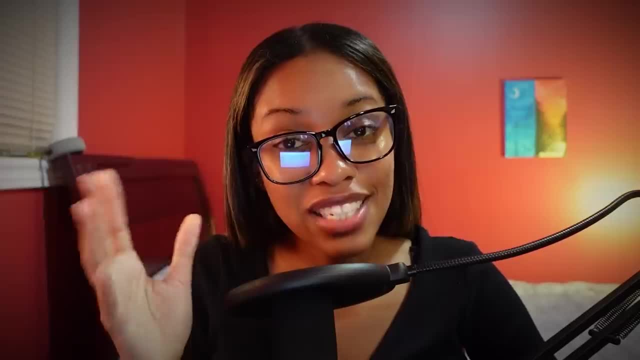 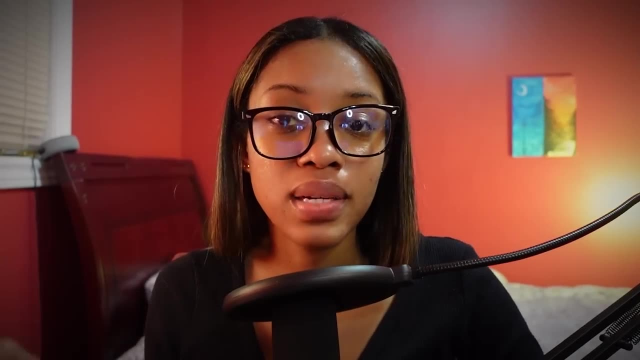 faceless videos using my best method. yet, And just so you know, this can be applied to any single niche. So the first thing you need to do is get video ideas. You can go about doing this in two different ways, So the first way would be simply coming up with the ideas yourself. 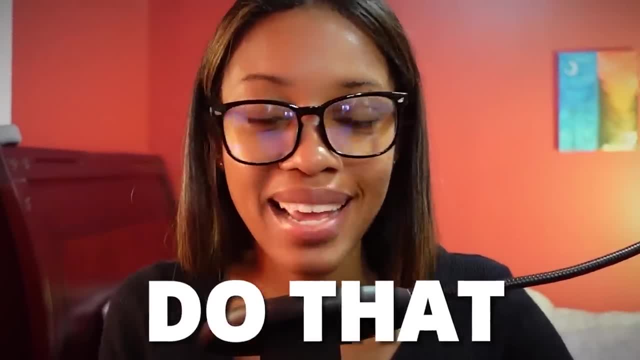 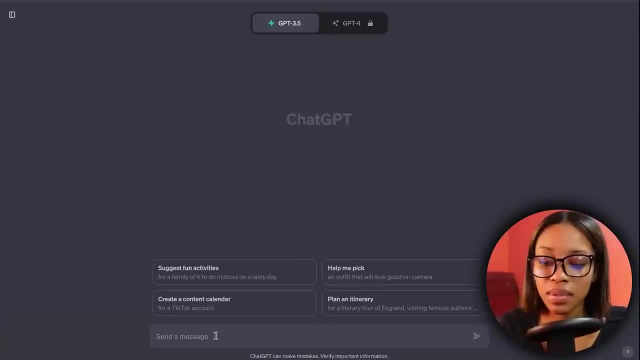 If you have that creative mind and you could think of stuff, great job, do that. If not, don't worry, because the second way you can go about getting video ideas is by coming on over to ChatGPT. Now, once on ChatGPT, you're going to ask it for this prompt: Give me 20 simple video. 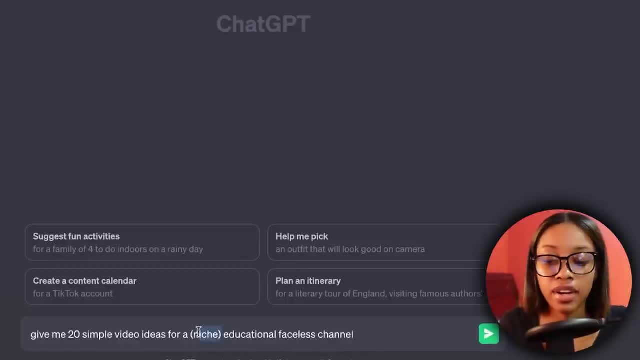 ideas for a niche, educational, faceless channel, And over here all you want to do is insert your niche. So this is the first way you can go about doing this in two different ways. So the first way you can go about getting video ideas is by using ChatGPT, So we would simply replace this. 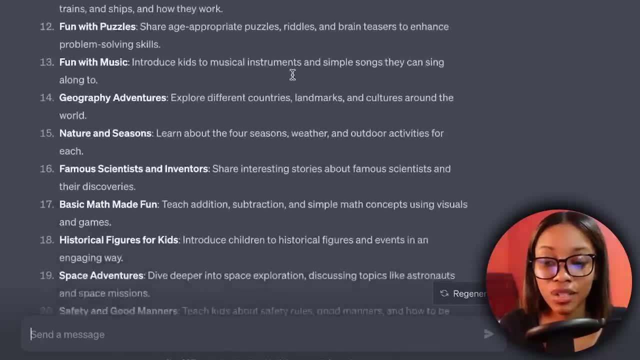 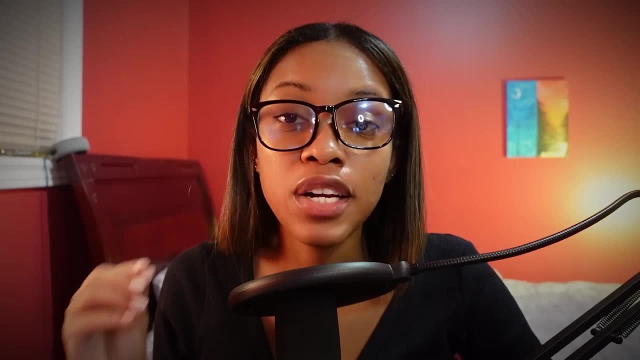 with kids and hit enter And, as you can see, it has gone ahead and given us 20 wonderful ideas. Now, once you have your video ideas, the second thing you need to do is come up with the video scripts. Now you can go about doing this in two different ways Now. the first way would be coming. 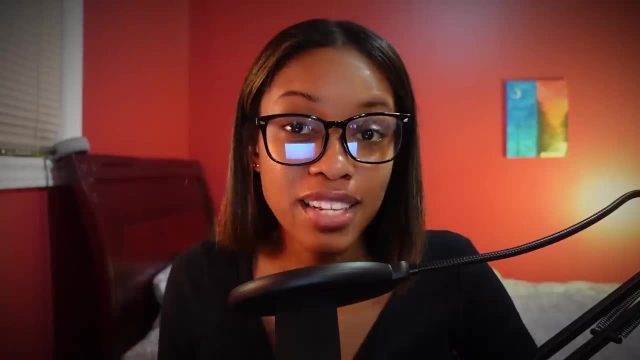 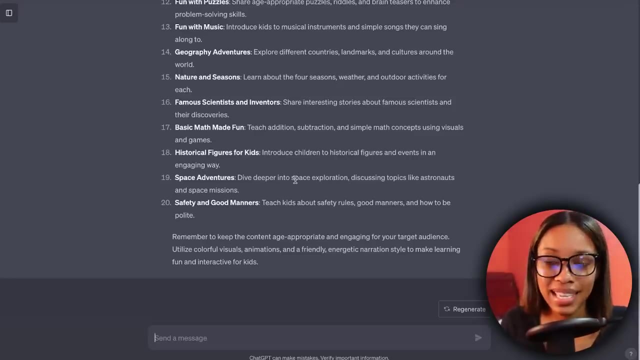 on over to a Google Doc and writing the script yourself. If you can't do that, go ahead to do that Now. if you can't come up with your own scripts, the second way you can go about getting your script is by using once again ChatGPT. Now, once on ChatGPT, you want to ask it for this prompt. 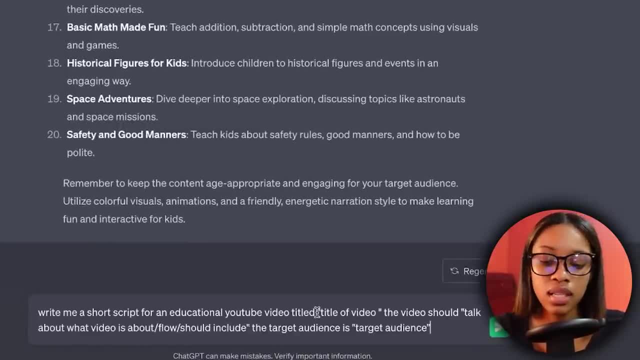 Write me a short script for an educational YouTube video title, And then you're going to insert the title of your video And then it says the video should. And then, over here, what you want to do is talk about what your video would be, about what you want it to include: the flow of. 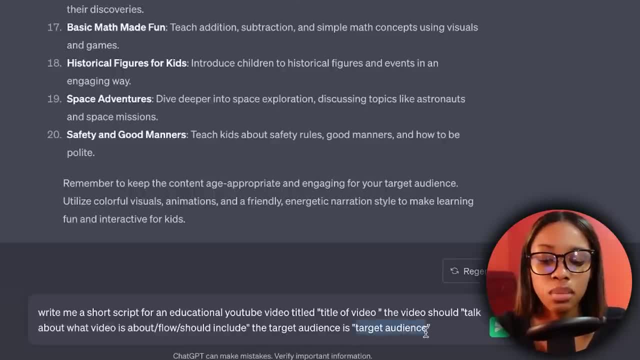 your video And then the target audience is, And then you simply insert your target audience. So in my case, this is how I would fill this out: Write me a short script for an educational YouTube video titled Name the Fruits. That would be the title of my video. The video should- and here I said: 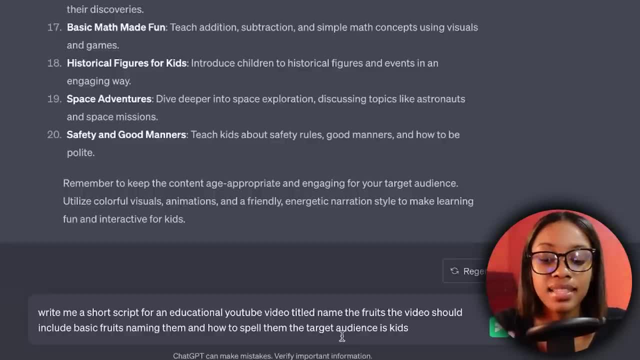 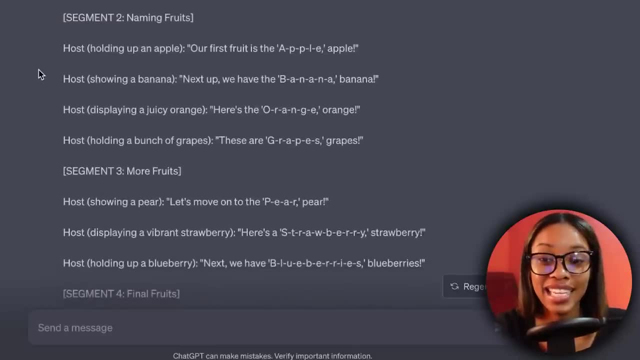 include basic fruits, naming them and how to spell them, And then the target audience is kids. That's how simple it is to use this prompt. Then hit enter And now, as you can see, ChatGPT has gone ahead and given me a great script that I could use for my video. So, whether you decide to, 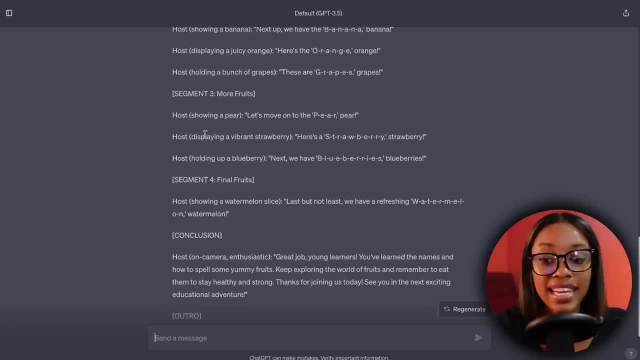 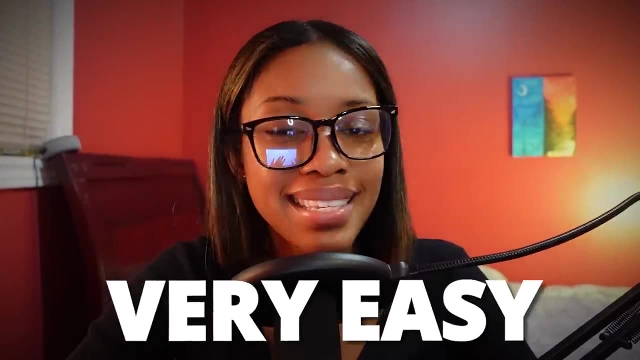 use the ChatGPT script, create your own script or edit this script to fit your needs better. once you have your script, it's time to move on to the next step. Now, for the sake of this tutorial, to make it very easy and digestible, I've gone ahead and created my own script And, as you can, 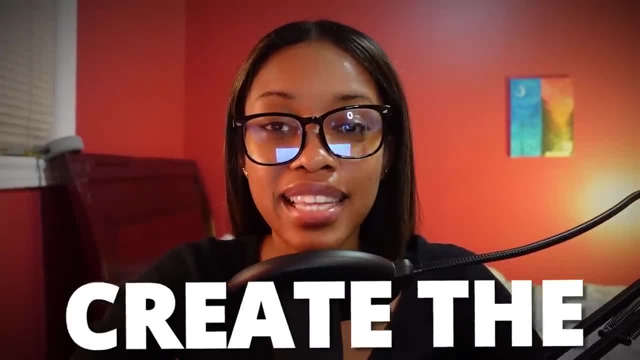 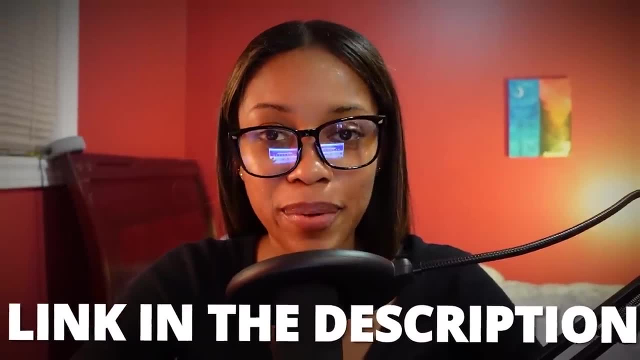 see, it's very simple and to the point again. So now the next thing you need to do is create the characters for your animation. Now, in order to do this, we're going to be using Canva. You can find the link for Canva in the description below. Now, once on Canva, what you want to do is come on over. 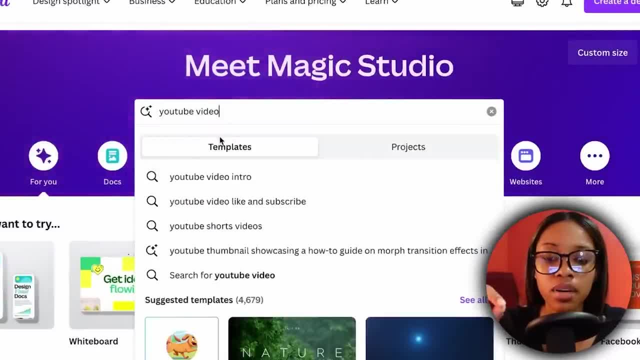 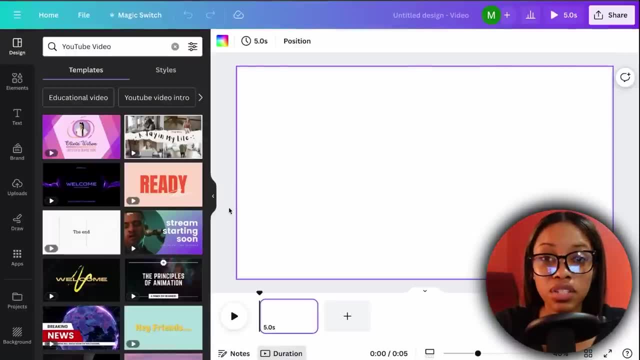 to this section and then simply do a search for YouTube video and then hit enter And then, once you've done that, you're going to click this one which says create a blank YouTube video. And now it's going to take you to this scene where we can begin creating the characters. And I swear to you, 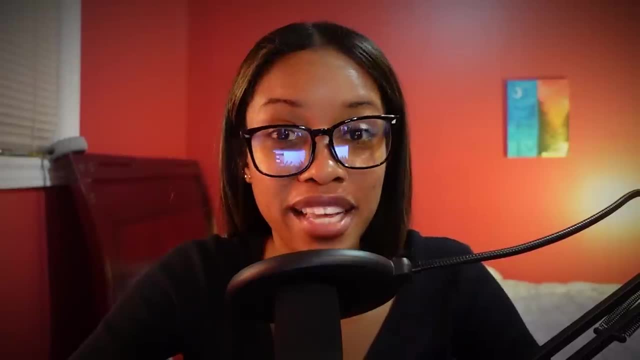 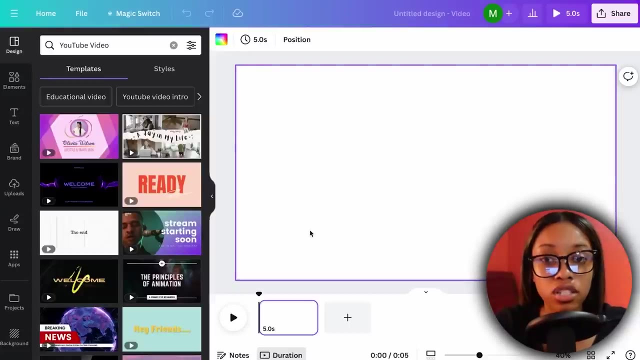 this part is super easy, but it's also super fun because you get to be really creative. So now our video is about fruits. I have three fruits: a pear, an apple and an orange- So the first thing I would need to do is get these elements Now. in order to do this, I would come over to this section, where 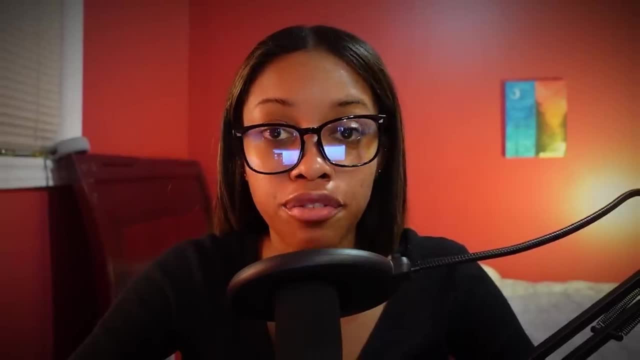 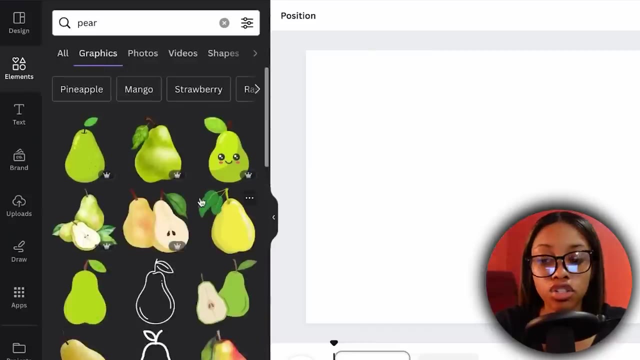 it says elements. Now, once on elements, I can go ahead and search for the fruits I want. So the first one is a pear. So I do a search for pear and then click onto where it says graphics, And then you could scroll through all these options and choose whichever pear that you prefer. So I'm 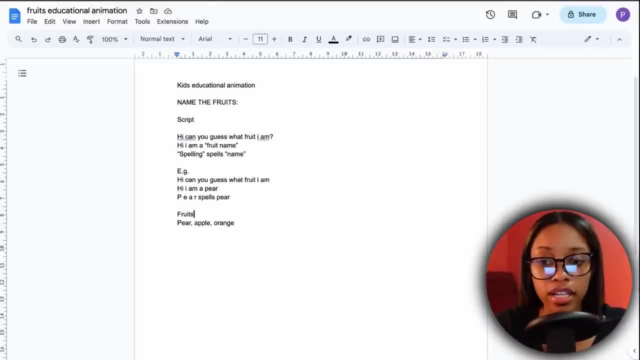 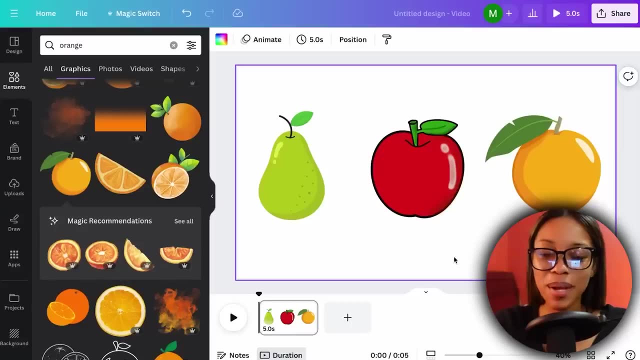 just going to choose the first one that I see. So my other elements were the apple and orange, So I'll do the same exact process to get all my characters. So now, as you can see, I have all three of my characters. Great job, But this isn't really giving anything special. It just looks like. 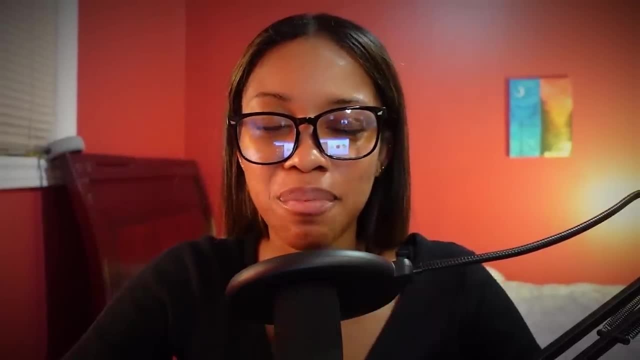 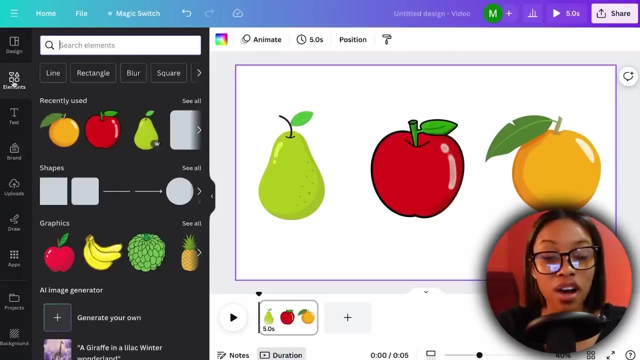 three fruits. Instead, we need to actually try to bring them alive a little, make them look like actual characters. So, in order to do this, we need to give them some body parts. So what you'd want to do- ensuring that you are in the elements once again- you're going to go ahead and do a search. 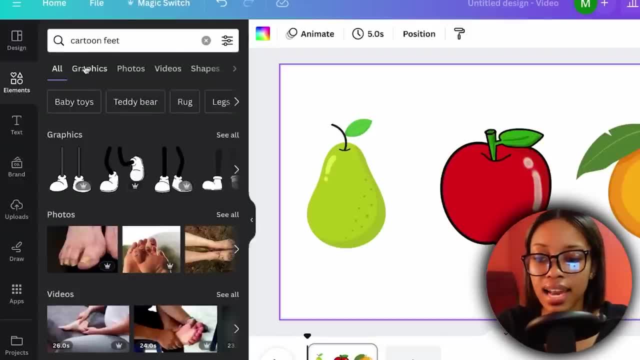 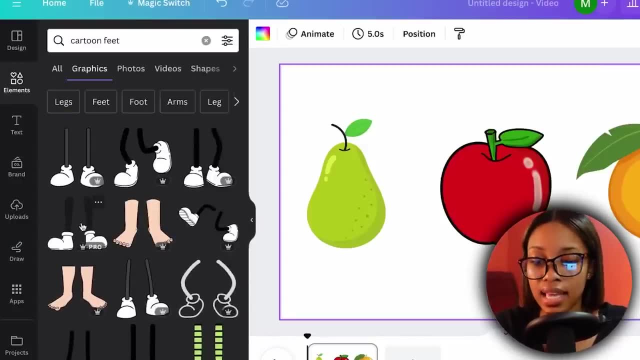 for cartoon feet and then hit enter, And then you're going to go ahead and do a search for enter. Once you've done that, click over where it says graphics. And now, as you can see, there's many different feet that we could choose from, So the one I recommend you use is this one And once. 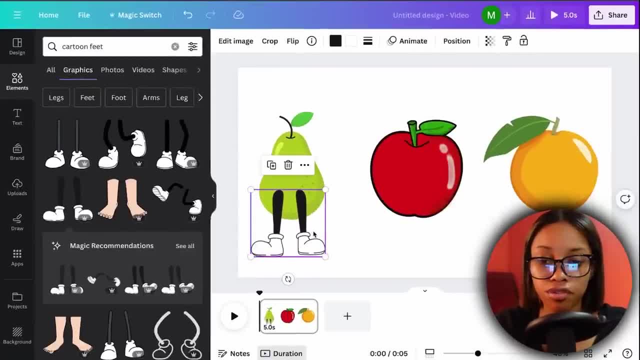 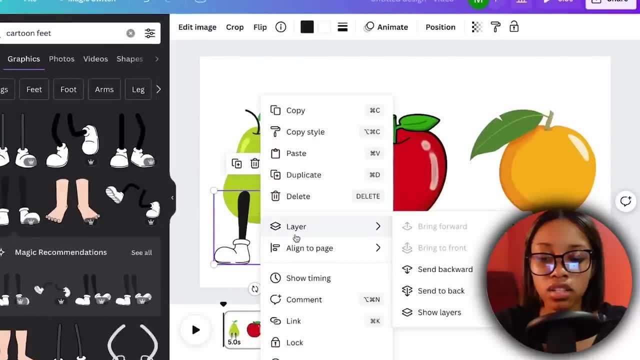 you've clicked onto it, you can now position it and adjust it onto your fruit character And, as you can see, it's in front of the pear. We don't want that. So in order to put it behind the pear, you want to right click onto it, click layer and then just simply click send backward. And now we. 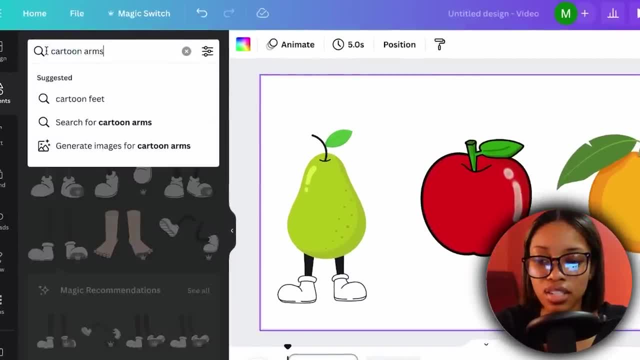 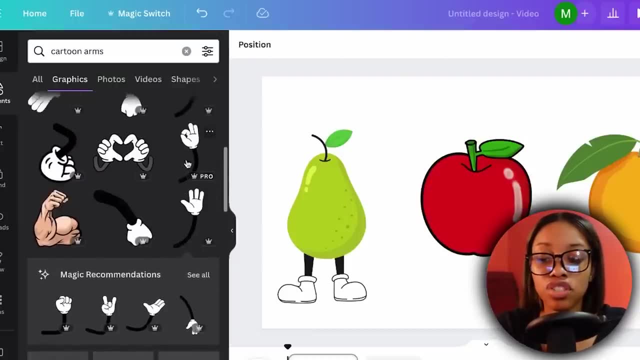 need to give it some arms. So in the search box we're just going to search the same thing, but hit enter. So, as you can see, there's many arms to choose from. So scroll through this and choose the one that you would like, And then, once you have it in, you simply need to adjust it onto. 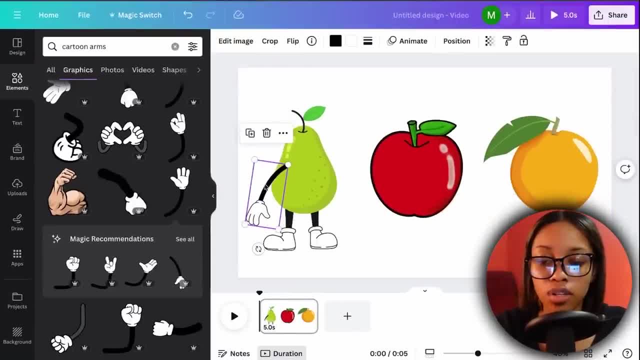 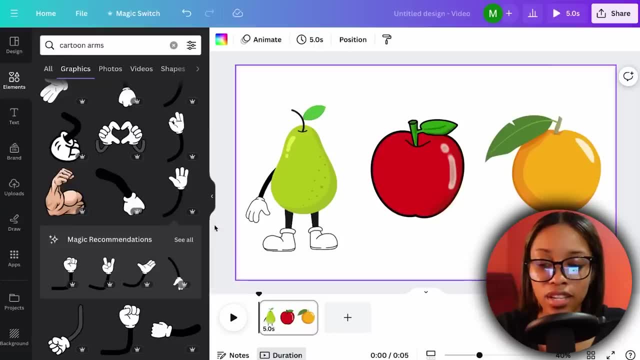 your character And once again it's at the front. We don't want that, So we're going to right click layer, send backward. It's coming together great. So we need to give him another arm. In order to do this, you click onto this one, right click, duplicate. Now we have two arms. 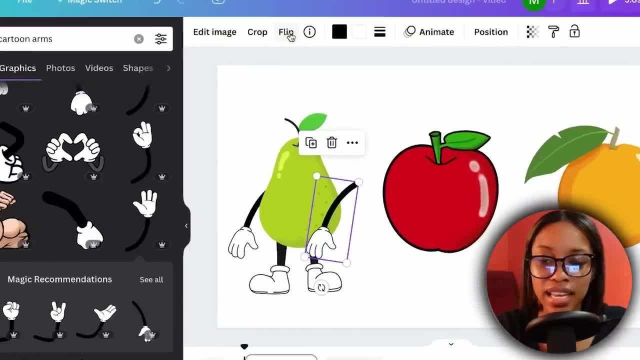 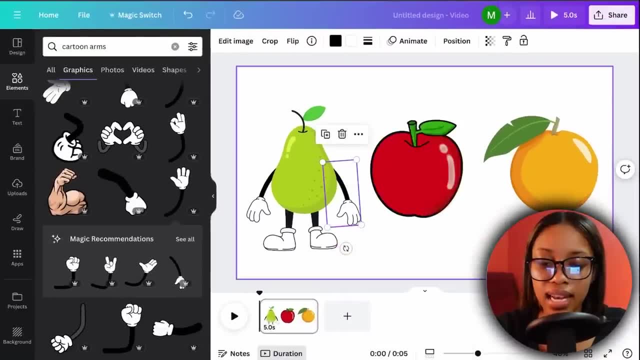 but it's a little bit sideways. Don't worry, that's an easy fix. Simply click, flip horizontal, and then there you go. You can now adjust it and then send it behind. And look at this: the pear is already looking way better, And now the last thing we need to do is give him a 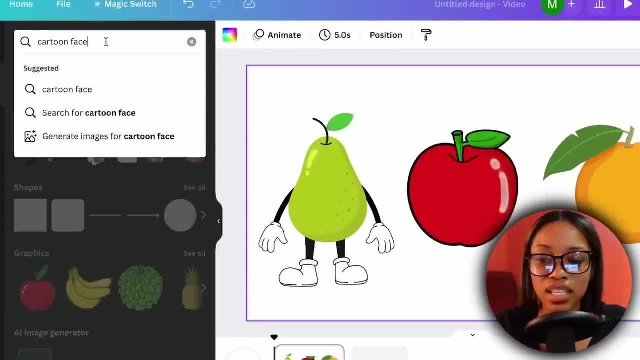 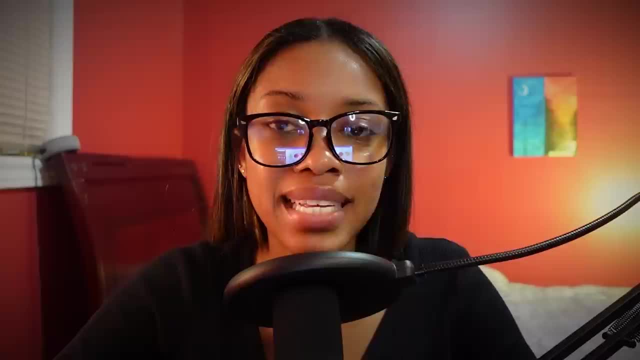 face. In order to do this, we're going to come to elements and then do a search for cotton face, click graphics And then, as you can see, there's lots of different faces to choose from. So you just scroll through this and then choose the one you like. And once you find the one you like, 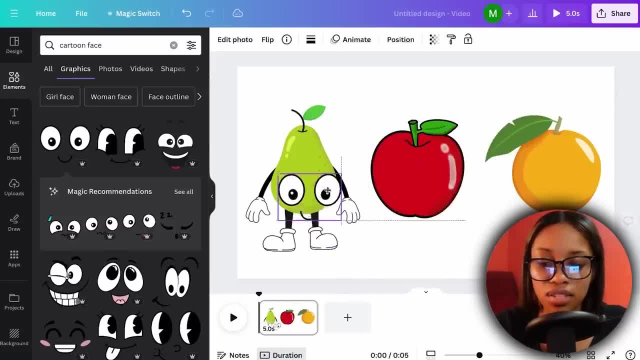 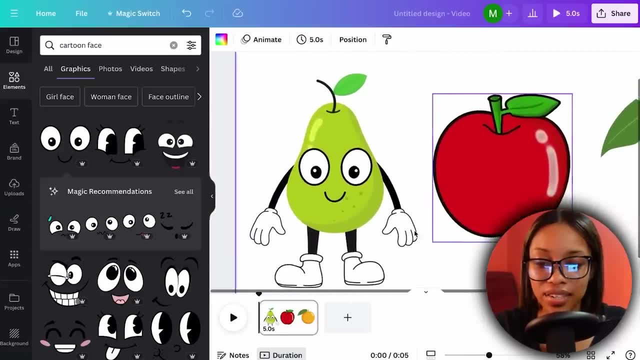 you simply click onto it and then you just adjust it to fit onto your character, And there we have him. He looks so cute. I think he looks adorable, And that's how easy it is to create your character. And then there is one last thing you need to do to him. As you can see, his legs are. 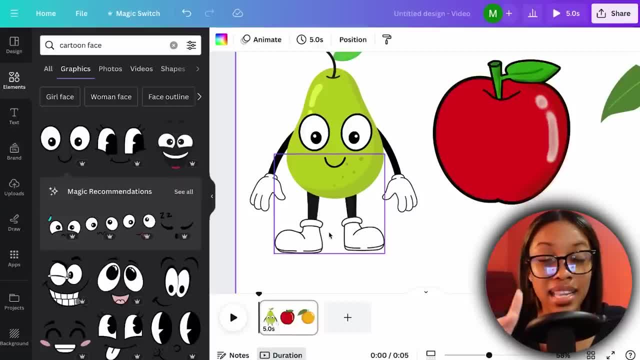 both facing opposite directions. You want them to face the same direction, and that'll come in handy when we're going to animate him. So just trust me, I've never said you guys wrong. So in order to do this, the first thing we need to do is get it to be one leg. So you'd want to click. 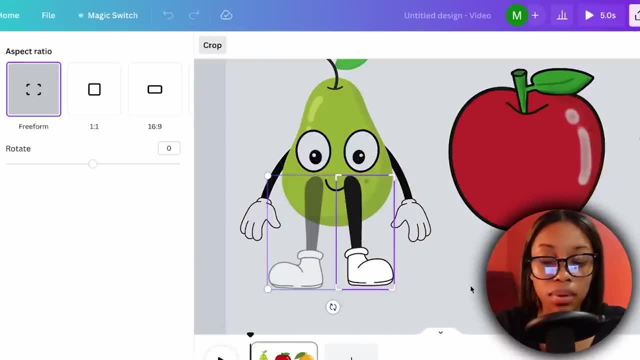 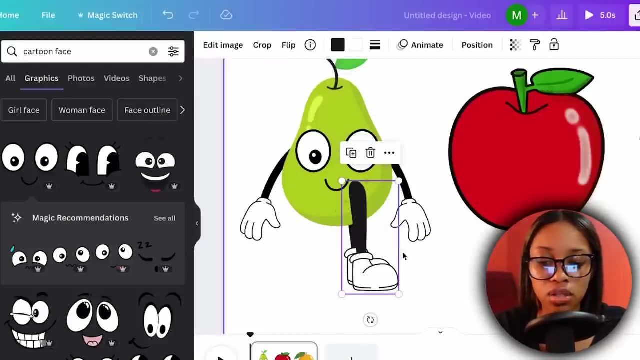 onto this click where it says crop, and then simply just crop it to be one leg. Now we need to give him a second leg. In order to do this, you're going to right click onto the same same leg and then you're going to click duplicate And then now, as you can see, he has. 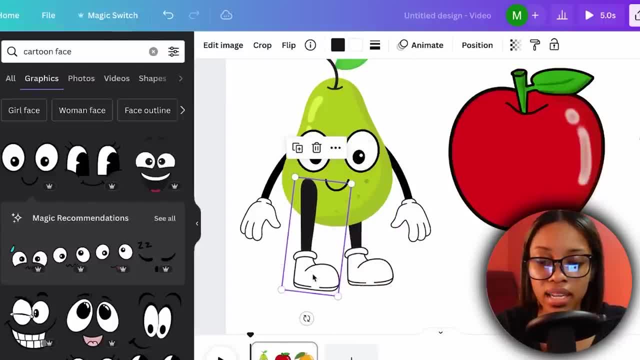 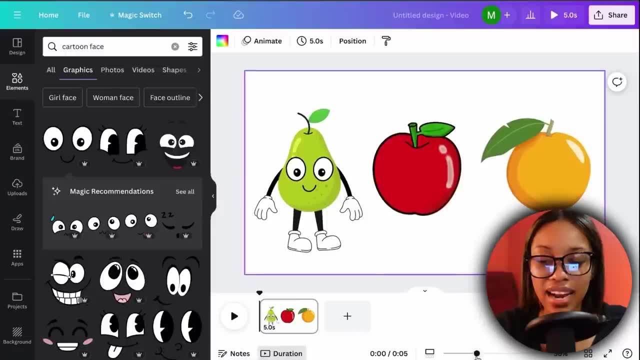 two legs. You want to bend it a little so they don't look too weird, And then you're going to right click again and then you're going to send it to the back. So now, as you can see, our first character is done, And now you need to do the same thing for all your other characters. But whoa. 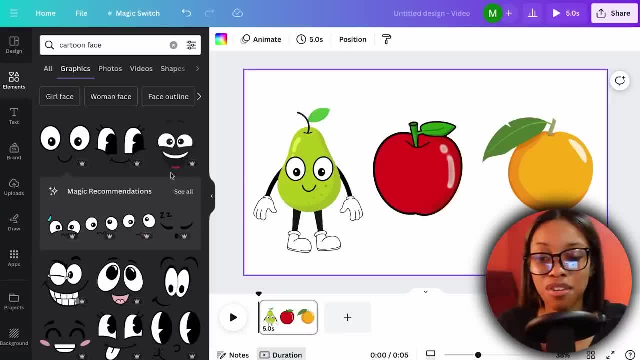 whoa, whoa. don't worry, You do not have to go and do this whole process and find all these things again. unless you want to, You can simply duplicate it. What I mean by that is this: You're going to. 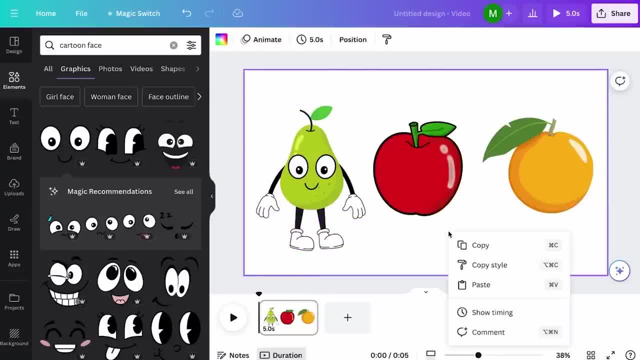 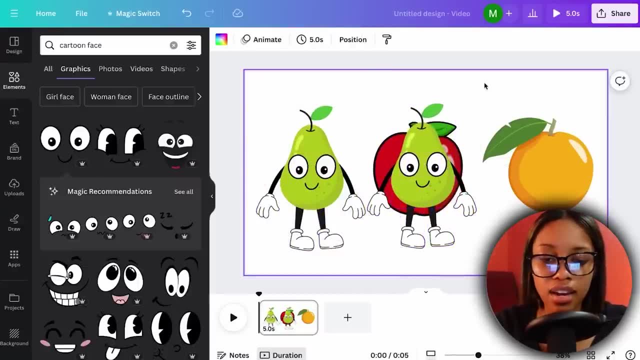 our entire pair, and then you're going to copy it. and then you're going to paste it- As you can see, we have two of them- And then you're going to put him over your second character, Then you're going to click out of it. Then now you're going to click onto the pair and delete him, And now 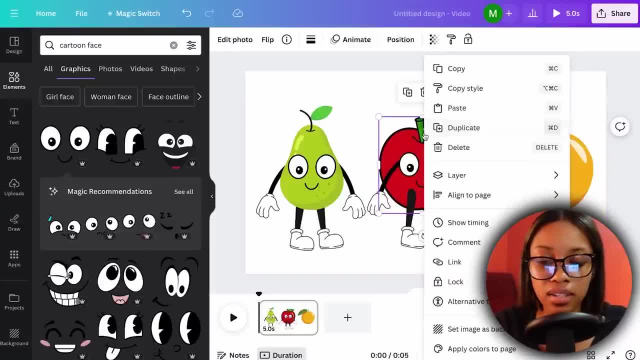 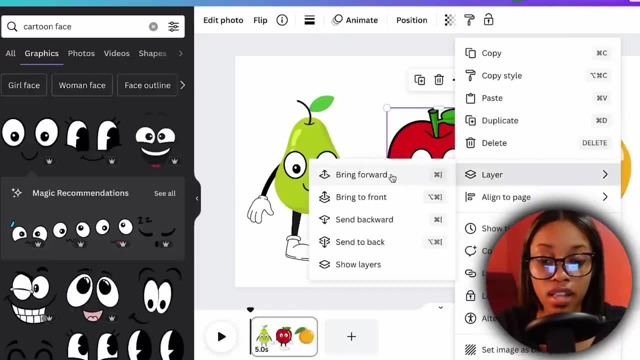 as you can see, we're mostly done with our apple. All you need to do now is click onto the apple, click where it says layer, and then click bring forward, And then you want to keep bringing it forward until it's in front of all the legs. And there you go. It was that simple, So from here. 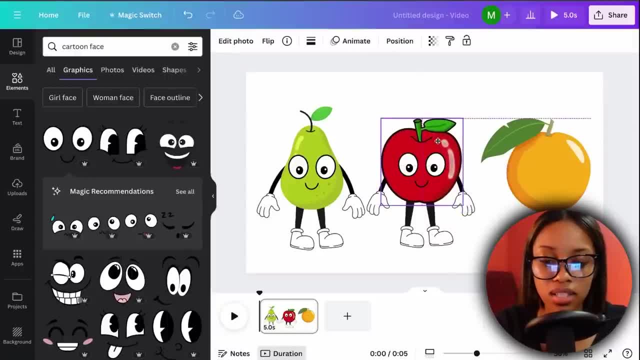 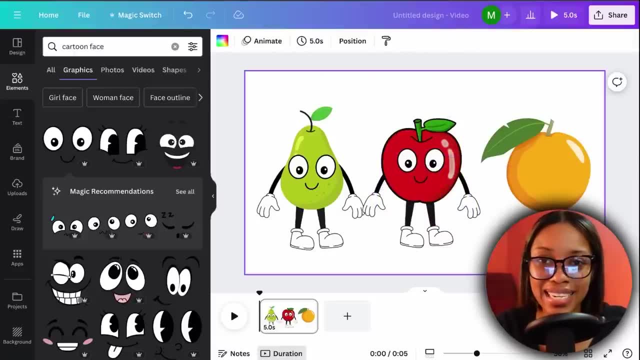 all you'd want to do is maybe just adjust the sizing So it's not too big or not too small, Readjust different aspects of it And now, just like that, within five seconds later, I had my second character done. So this is the process you 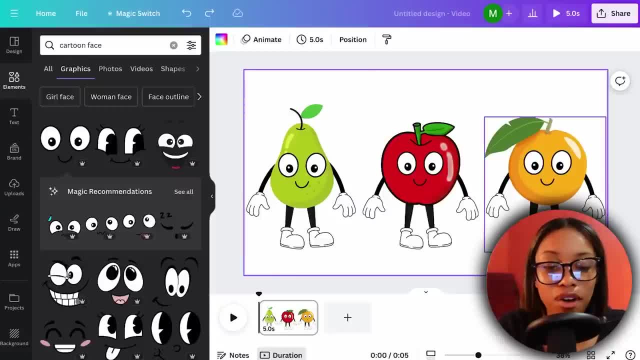 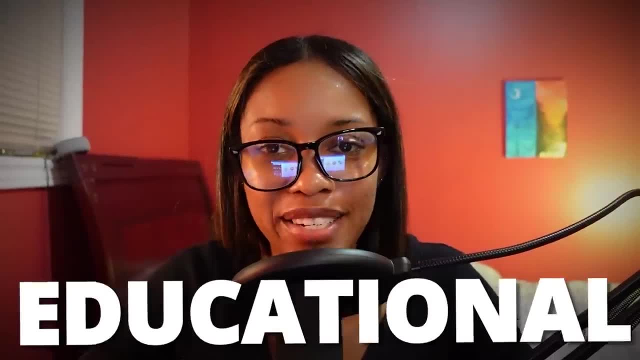 want to do for all of your characters. And now, as you can see, I have all three of my characters done, So now I can go ahead to further edit them to be the perfect characters that I would want in my educational video. And now, once you have your characters done, it's time to download them. 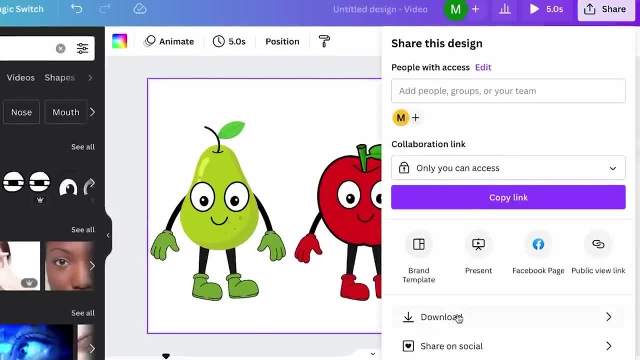 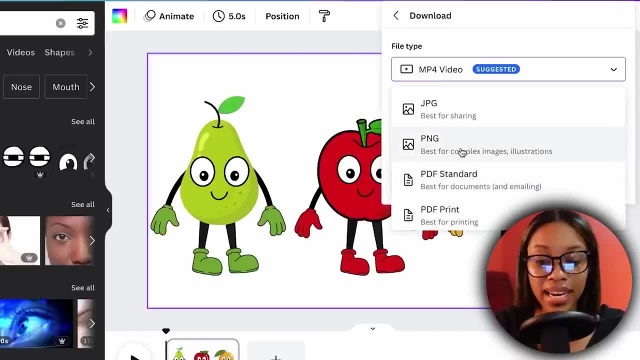 In order to download them. you want to click onto where it says share and then you're going to, And then you don't want to download it as an mp4. So you're going to click onto this and then you're going to scroll up and click PNG and then you're going to go ahead to hit download. 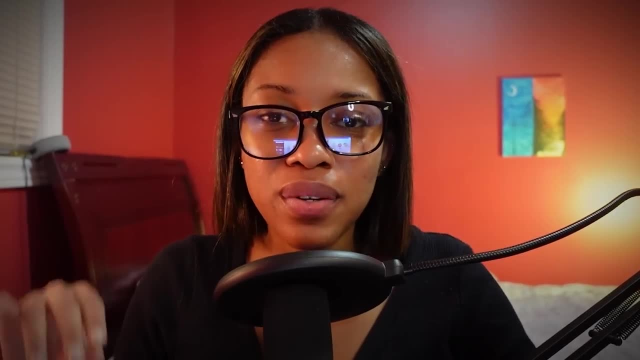 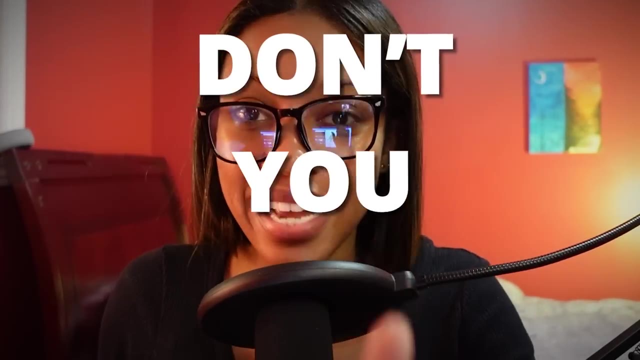 And now it's time to move on to the next step. So now the next thing you need to do is animate them. You're going to bring these characters to life, And before you say, oh, nevermind, this is where I click off, Don't you dare, Because the method I'm going to show you requires no skills whatsoever. 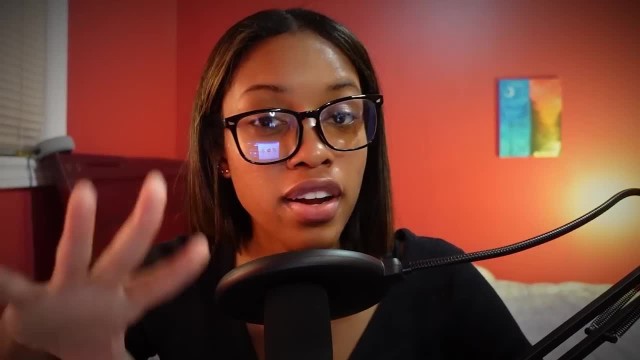 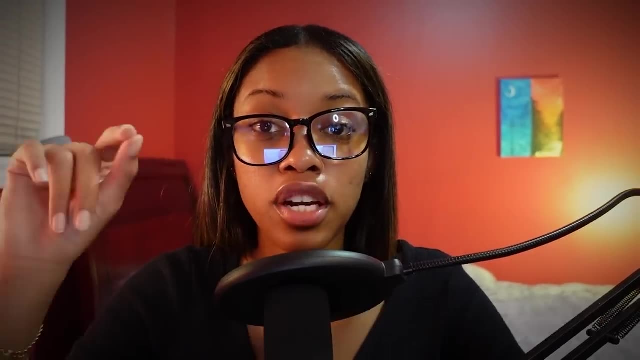 and it's literally done by a few clicks of a button. So, in order to bring them to life, we're going to be using this tool called Animator Drawings. I'm going to leave a link for it in the description. Now, once on. 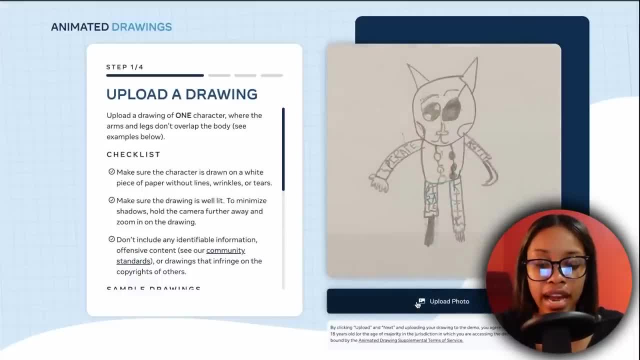 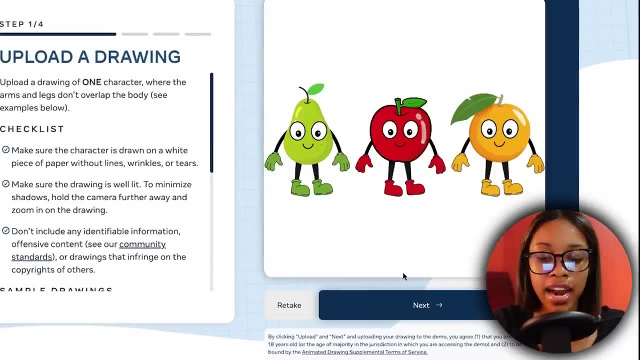 Animator Drawings. it's going to take you to this page And on this page over here, where it says upload photo, you want to upload the photo of the characters that we just downloaded from Canva, From here. you want to click next and then it's going to take you to this page where you now need. 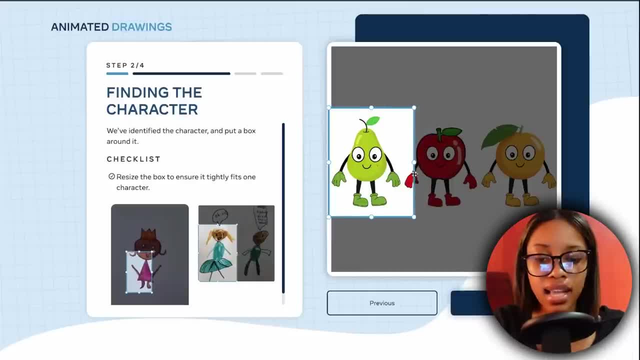 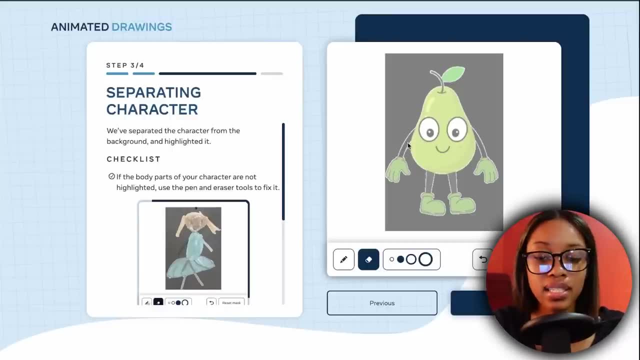 to select one character. So we're going to just adjust these lines and select our pair and then hit next And then, once you've done this, as you can see, it's going to take you to this page where it's now outlined our pair. Now you need to make sure that your entire character is actually 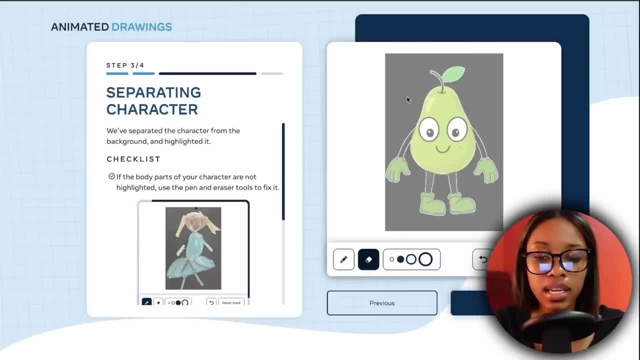 outlined like this: If there's a piece of the background in, you can click the erase button and then you can erase it- Now, we don't want to erase this, so let's undo. Or if there's a piece of it that's not in the lines, you can click on the draw button and then you can simply add it. 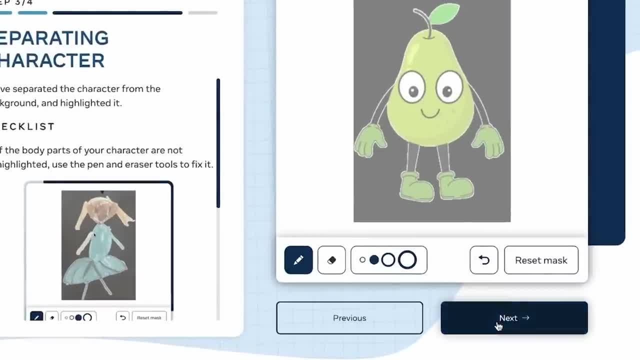 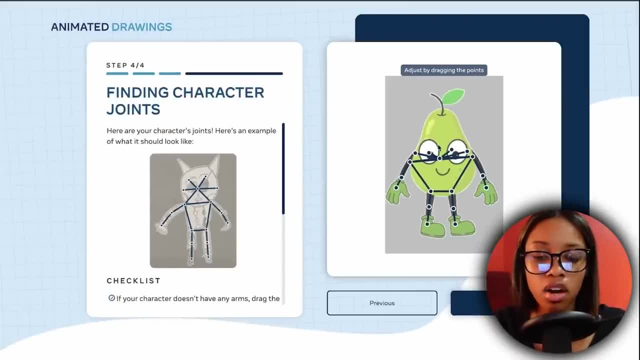 in by coloring like this, And then, once that part is done, you need to click next And then from here you need to adjust the main points on your character. It mostly gets this well, but if it's a little off, then you simply put your mouse on the circle and, as you can see here where it says: 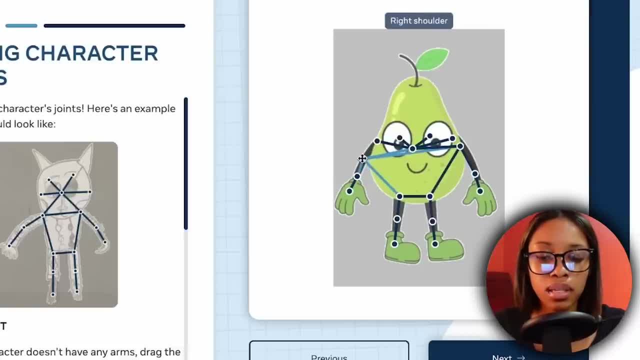 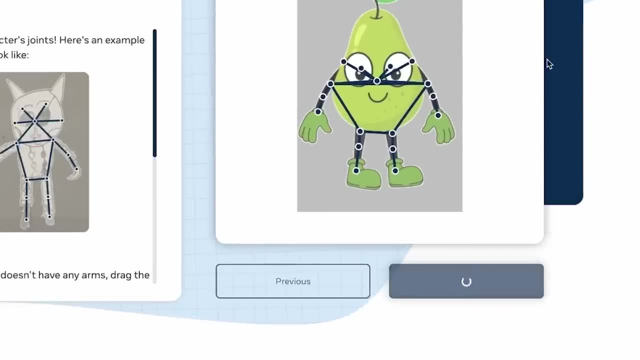 right eye. you'd put it on the right eye, So you just adjust it properly according to what it's supposed to be. Now, once you've done that, it's time for the magic. All you need to do is click next. Voila, look at this. Our animation is done. Look at him just running across the screen And 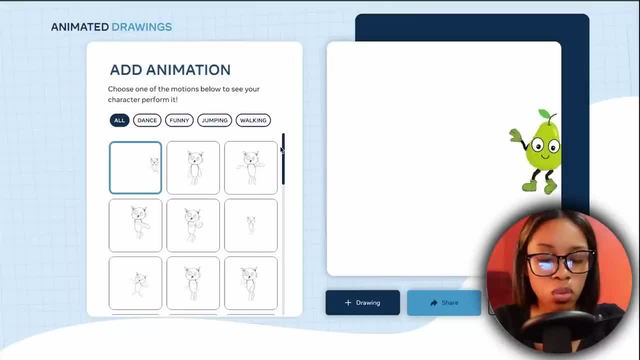 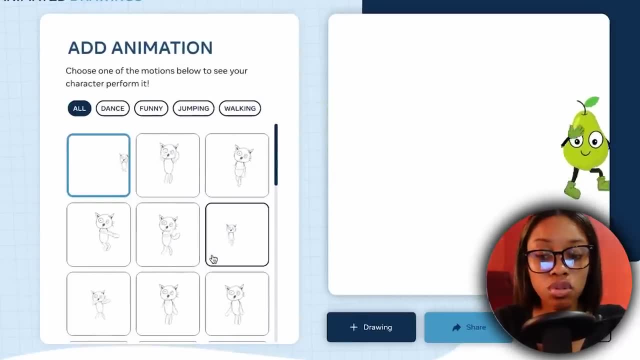 now, here's a great thing about this tool: We only had to do this once to generate him once, And then, on this side under here, where it says add animation, there's around 30 different animations, which would be more than enough for you to create an entire animation with practically any movement. 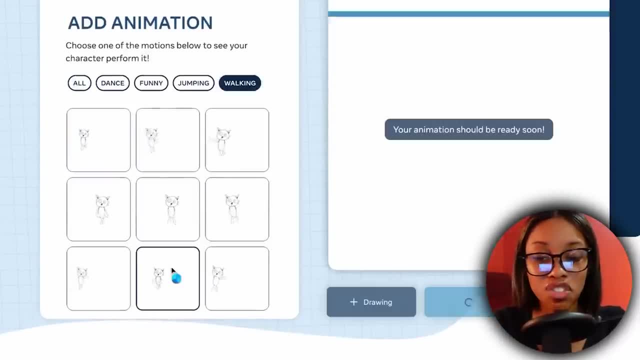 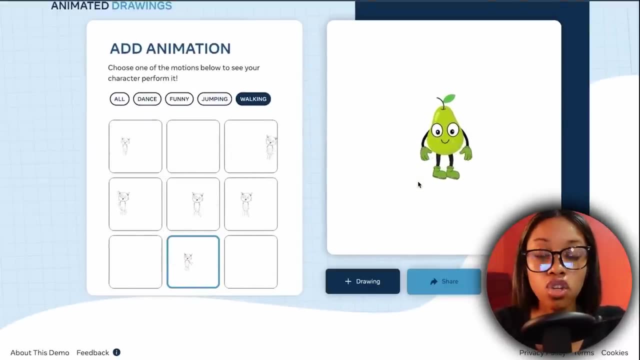 you could think of, And in order to change the animation, it's as simple as just clicking on the one that you want. And now, as you can see, here he goes And look at his legs. This is the reason why I said you wanted his legs to be facing the same direction, because if it wasn't, if his legs 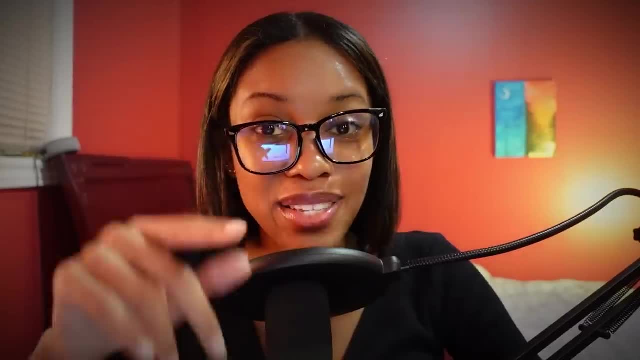 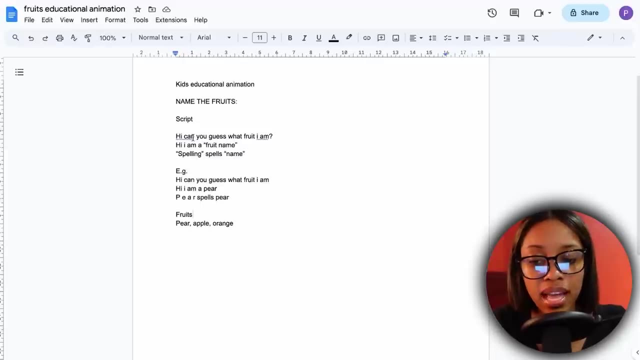 was facing the opposite way, he would be walking with his legs open. So that's why I told you guys to do that step earlier. See, I always have you guys covered. And then, from here, you would go to your script and then figure out the different movements that you'd need your character to do. 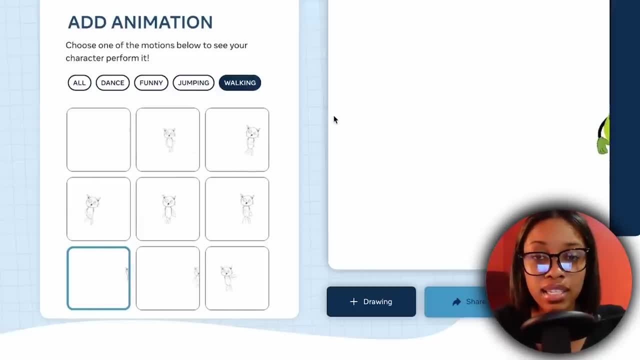 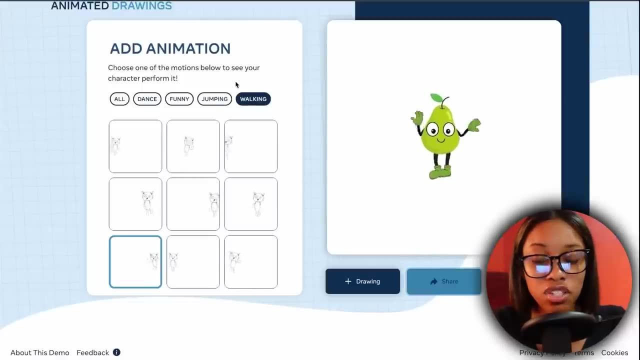 find it and then download it. In order to download it, it's very simple. All you need to do is click where it says share and then click download. So go back and forth from your script and animated drawings and just gather up all the different movements that you think you would need for your 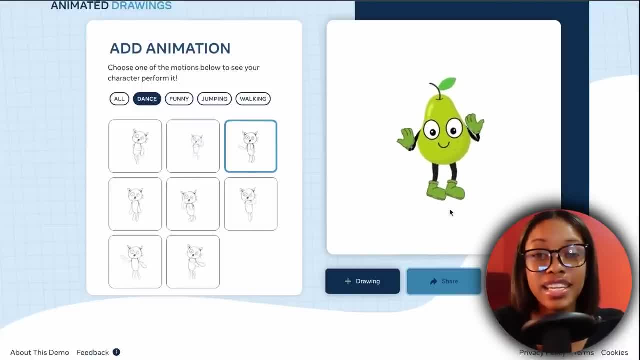 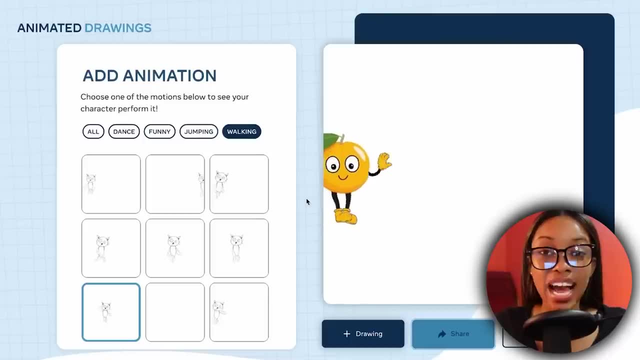 video And then, once you've downloaded all the moves for your first character, you need to go ahead to do this process for all of your characters. It's very simple to do, It doesn't take you long and it's completely free. Now, once you have all your characters, you can go ahead and 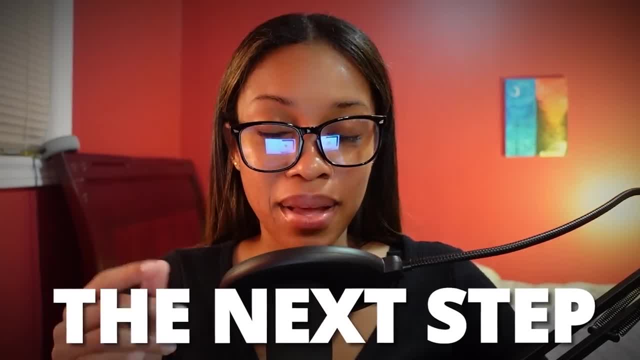 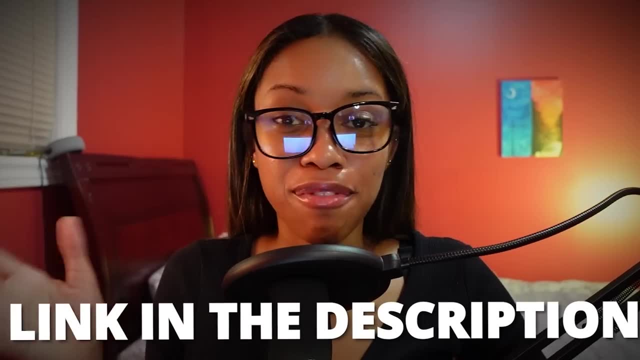 download it. It's time to move on to the next step. The next step would be getting the voices for your video. In order to generate the voices, we're going to be using Eleven Labs. You can find the link for Eleven Labs in the description of this video. But once on Eleven Labs, you want to? 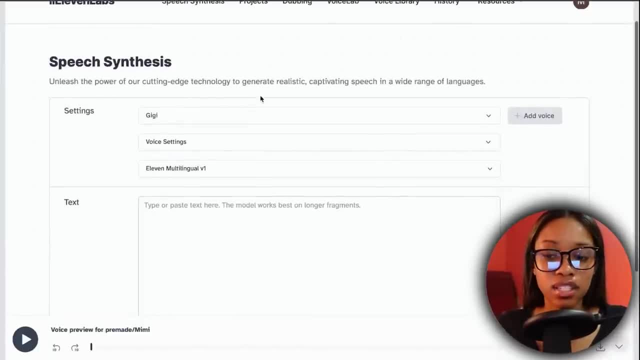 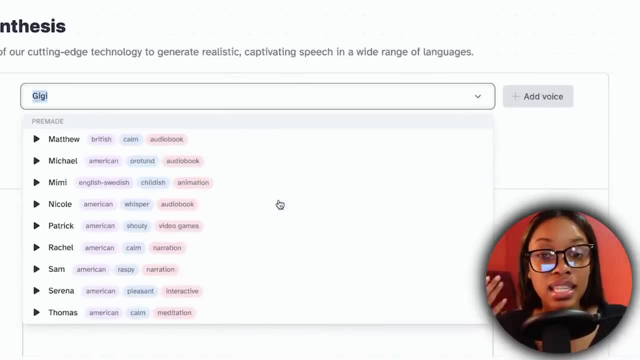 ensure that you are in the speech synthesis, The first thing you need to do is select the voice you want. In order to do this, you're simply going to click on the drop down arrow, scroll through all the different voices, listen to them and then just click on the one you want to use. So, for our 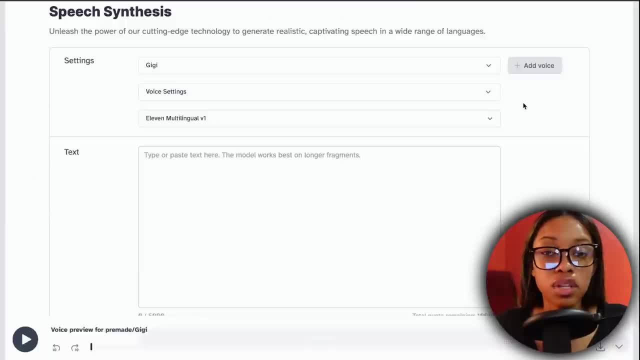 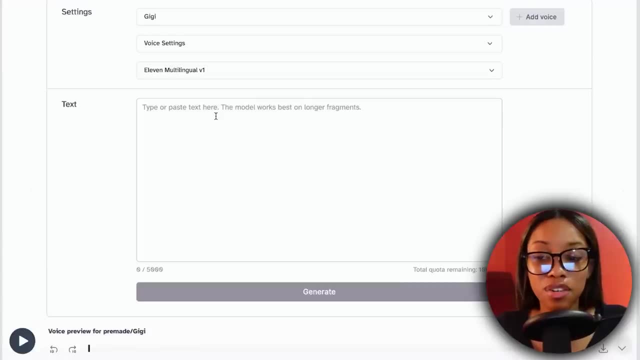 voice. I'm going to be using Gigi just because I love how she sounds. Now, once you have the voice selected, if you want, you can adjust the voice settings. You only do this if you want, It's not necessary. And then, once your voice is ready, you need to now add in the script of your animation: 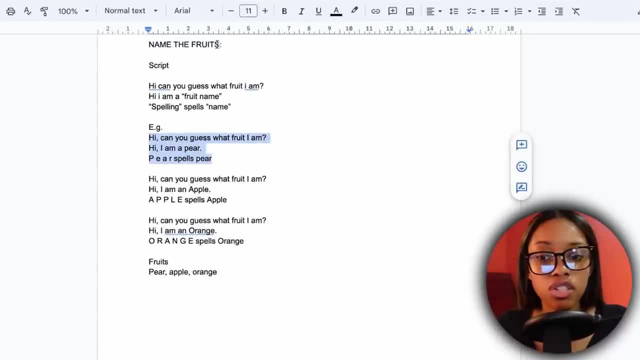 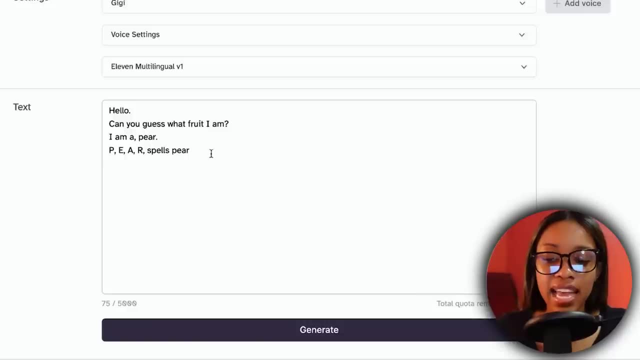 So I'm going to go ahead and copy the first section, which is what the pair is going to be saying. I'm going to come back over to Eleven Labs and paste it in And then, once you have imported your script, you want to go ahead to edit it with the correct punctuation so that your character can. 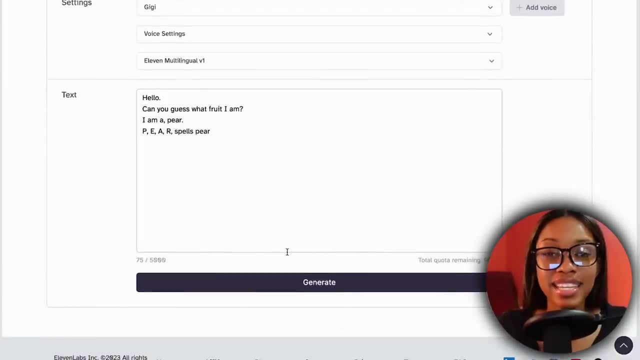 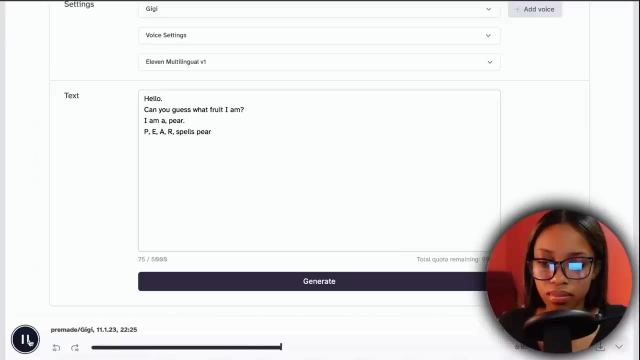 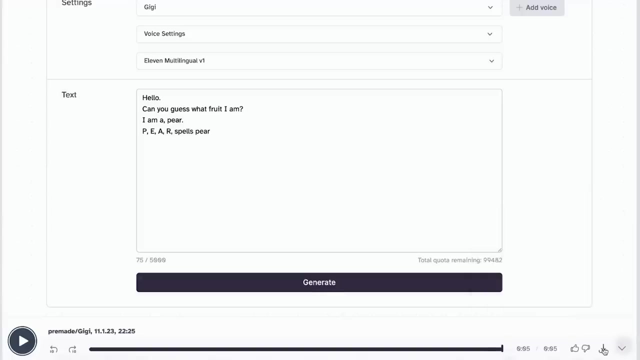 say it in the way you want it to be said. After you've done that, all you need to do is hit generate. As you can see, it's done. Let's just take a look at what this sounds like. Perfect. Once you've done that, you need to download your audio. In order to download it. 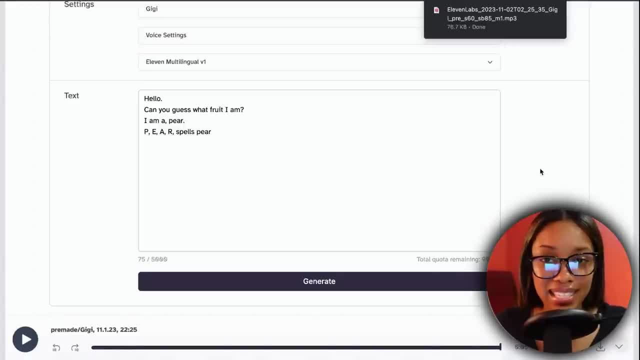 you simply come to this icon, click download and just like that it's downloaded. So now you'll go ahead to do the same thing for your entire scripts, And if you have different characters or if you want to use different voices, then for each new part of your 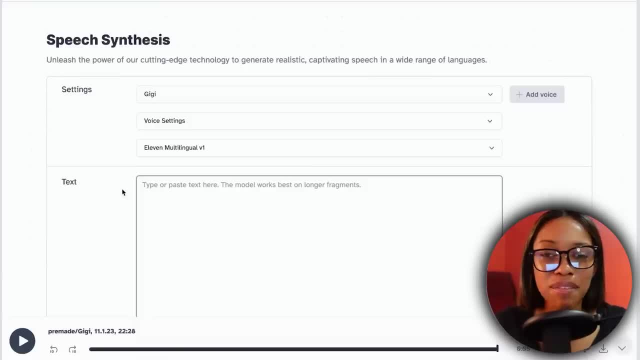 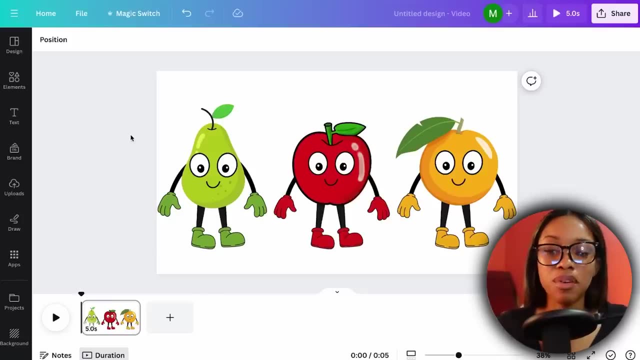 script. you simply change the voice and then generate it. And now, once you have all your voices downloaded, congratulations, Because now there's only one step left. In order to do the final step, you need to come back over to Canva. 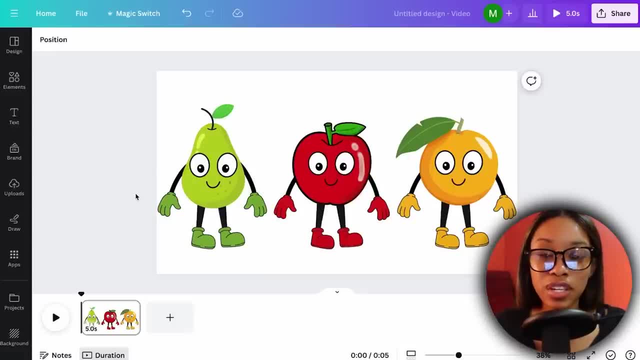 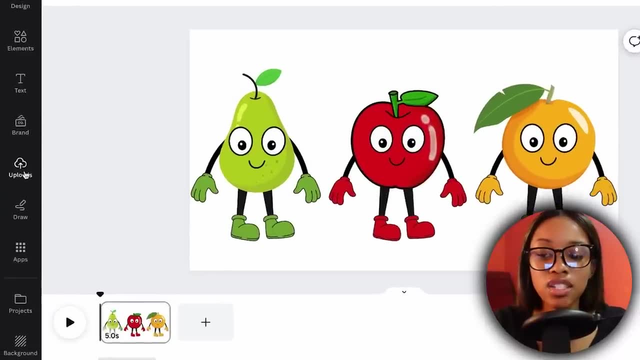 in the same section where you generated the characters, Because what you're going to do now is put everything together to generate your amazing animation. So the first thing you would need to do is click on to where it says uploads and upload all the files that you just downloaded onto Canva, So that'll be the voiceovers, and then 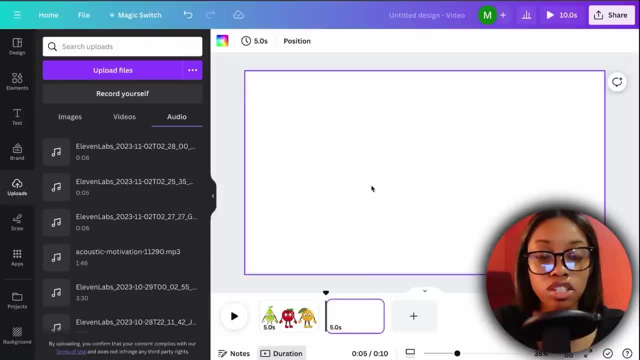 the animations. click over here where it says to add a page, so you can have a blank page to start from. so, from here, the first thing you need to do is get a background for your animation. so in order to do this, you'd want to come on over to elements and go to the search bar and then search for the. 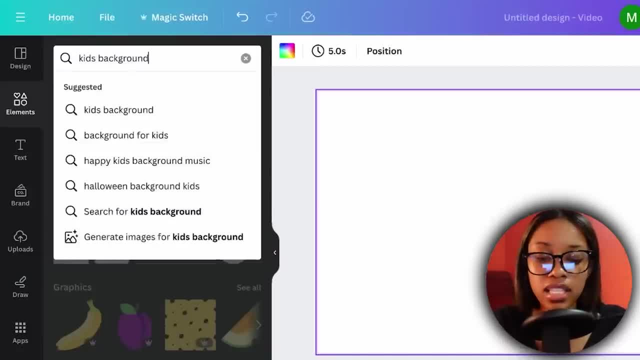 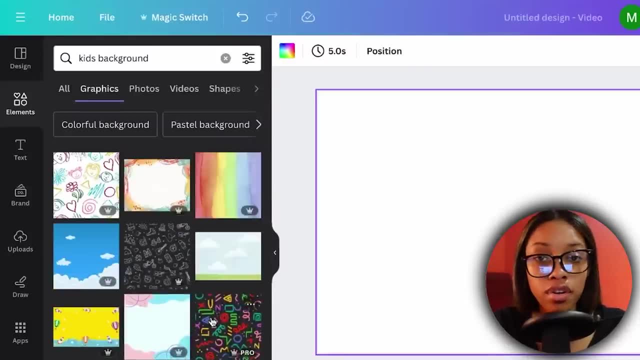 type of background you would want. so in my case, i'll simply search for kids background and then click on to where it says graphics, and then from here there's many backgrounds to choose from. so just scroll through and select the one that you like, and then from here you can adjust it to fit. 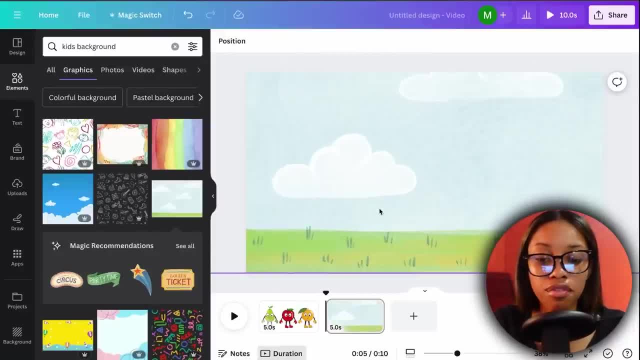 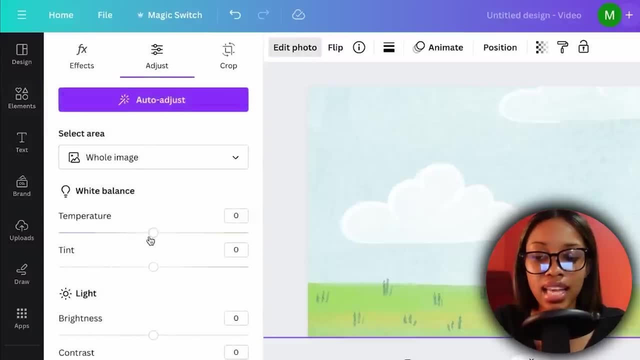 your scene better. then, once you have your background added in, feel free to adjust it even further to bring it more to life. by that i mean going to where it says edit photo, click and adjust and then adjusting these settings. so now that you have the background, you can now begin. 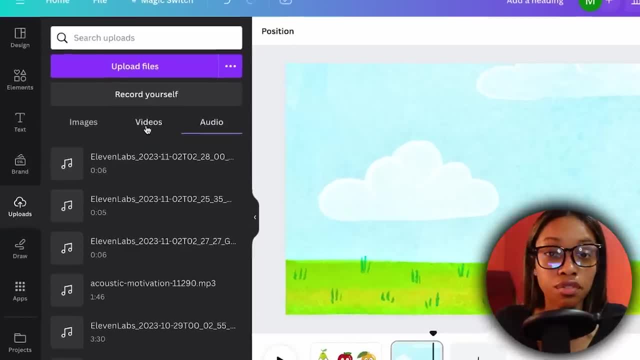 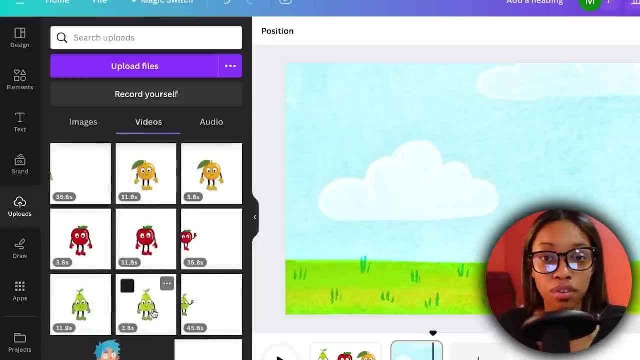 generating the actual scene. in order to do this, you want to first add in your character. so you're going to come on over to uploads and then go to videos and then select the animation that you want for your animation. so i'm going to go to videos and then select the animation that you want for. 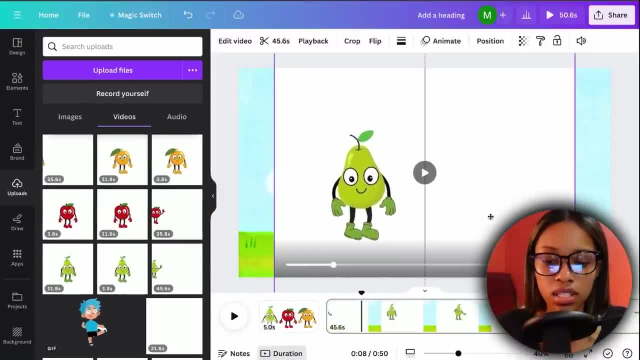 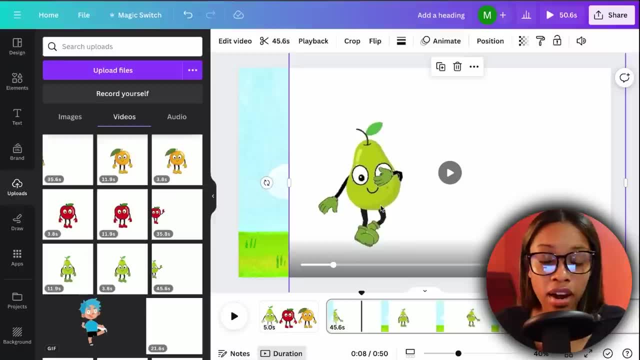 then you're simply going to click onto it and then you simply adjust the sizing of what you'd want it to be in your animation. now, as you can see, we can't just use it like this. it has this white background, so we need to get rid of it. in order to get rid of it, you simply want to click onto where. 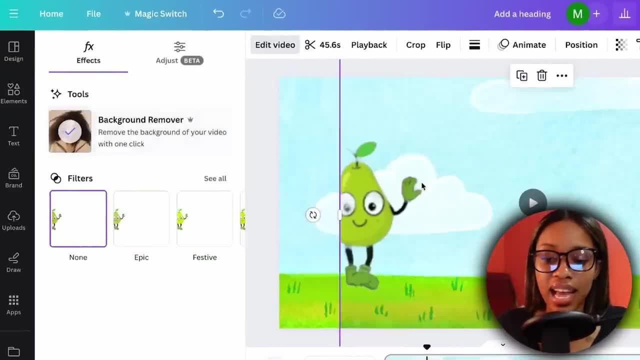 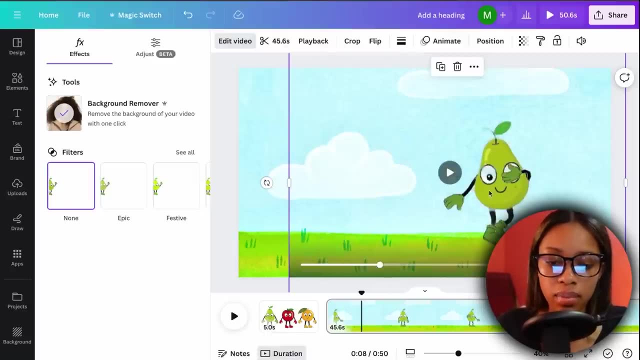 it says edit video and then click background remover and canva automatically removes a background for us. one thing i want you to do: notice: when it removed the background, it did do it a little bit spotty, as you can see. for example, the eyes are flickering and it's just because this tool is not 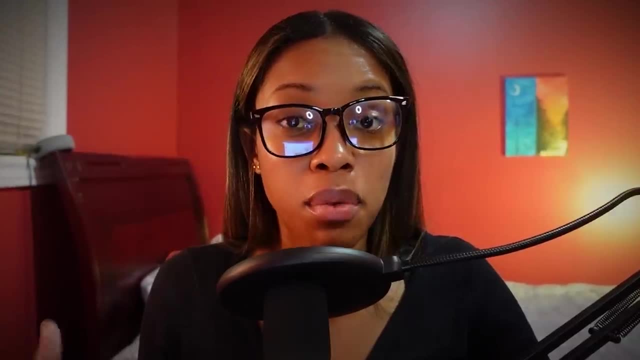 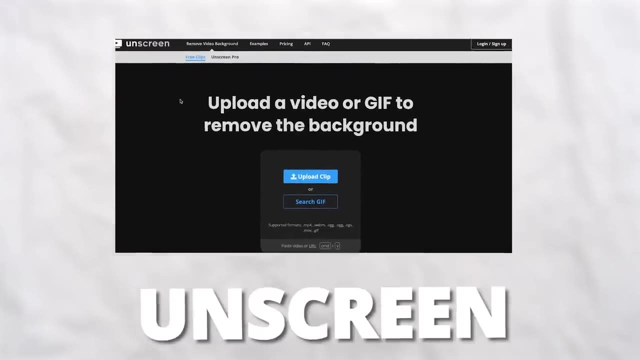 quite perfect. yet, especially when it's removing something from a white background, it's going to take out the eyes because it can't tell. but if you want to avoid this, then you can use this tool called unscreen. but just keep in mind that you do have to pay for it. so the choice is yours, but once 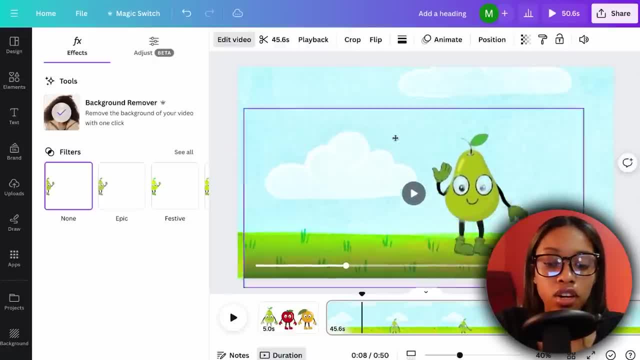 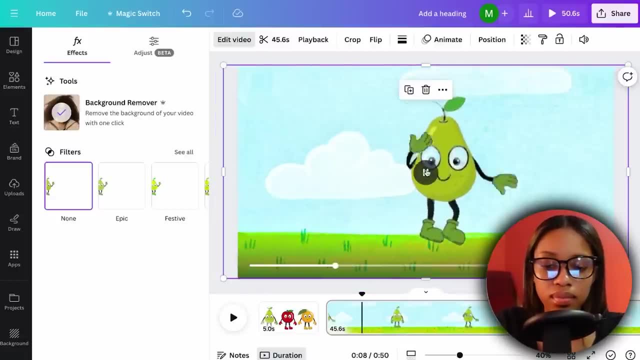 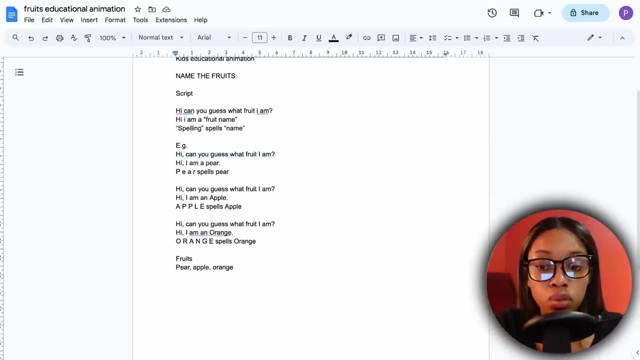 you have your video on your scene. you can now go ahead to further crop it and edit it to better fit the background. so now this is what we're working with and then, from here, what you want to do is take a look at your script and figure out what your character is saying, what they're doing. 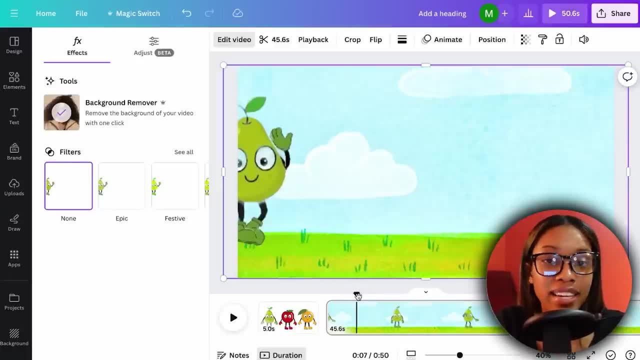 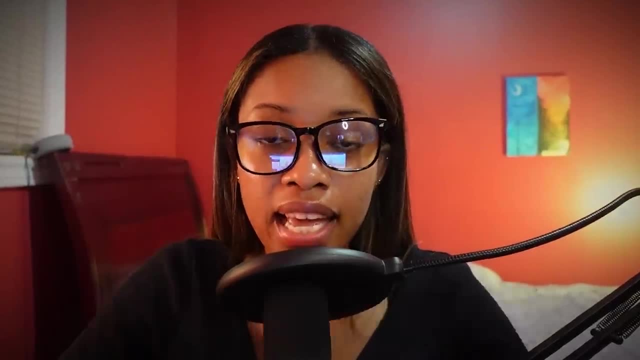 and then you want to crop and adjust your animation accordingly to that, and now, as you can see, we're mostly done with the first scene. but from here you need to make it more visually appealing. in order to do this, you'd want to add in the text of what your character is actually. 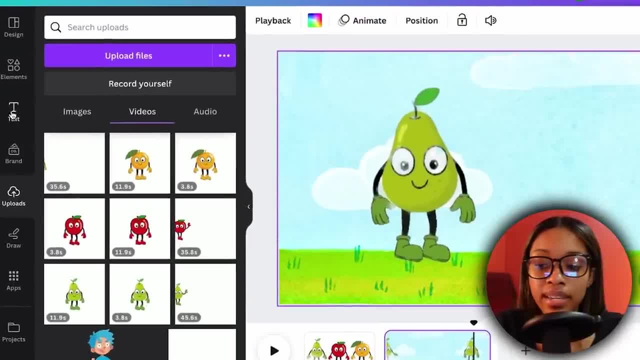 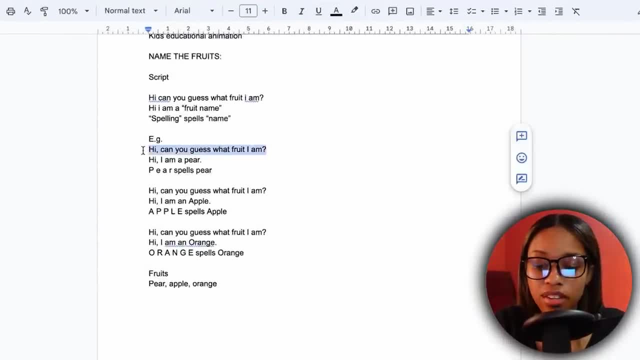 saying so in order to add in the text. you want to click onto where it says text. click on to add a heading. simply expand the sizing of this. go back over to your scripts, copy your script and then come back over to canva. delete this, paste it in and then, once it's in, you want to go ahead to. 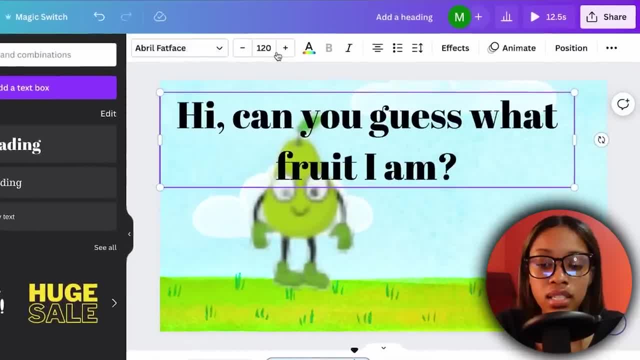 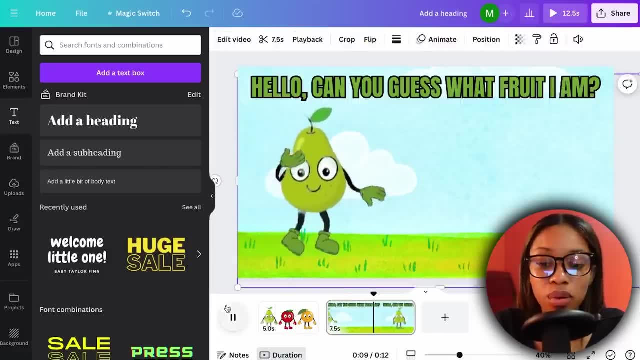 further adjust it to better fit your scene. you can adjust the text font, the sizing, the color, the effects, the animation. you do it however you feel like looks best. and now, voila, this is what we're working with so far. so now the next thing you need to do is add in the audio that your 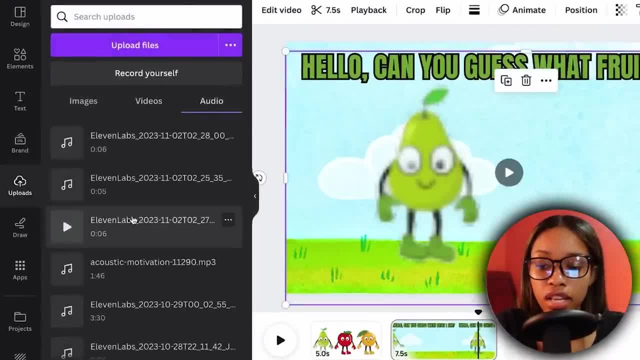 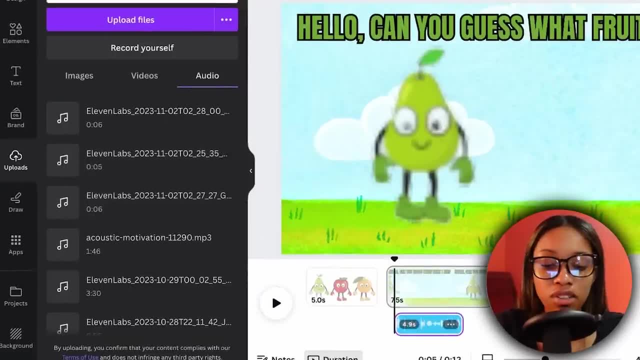 character is saying so you're going to go to uploads, click audio and then ensuring that your playhead is where you want the audio to start. you're going to then simply click on your audio now, just like that it's going to be added in, and then, once you have your audio added in, you want to. 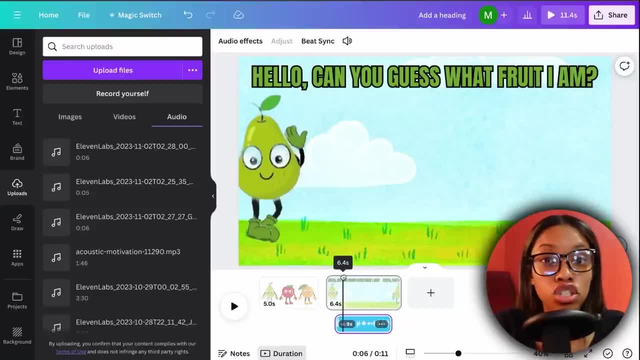 listen to it and see where the audio for that particular scene stops. so in my case, it ends out about here. so once you get to that point, you need to split the audio so that you can have the second part. in order to split it, you simply want to right click onto the playhead where you want it. 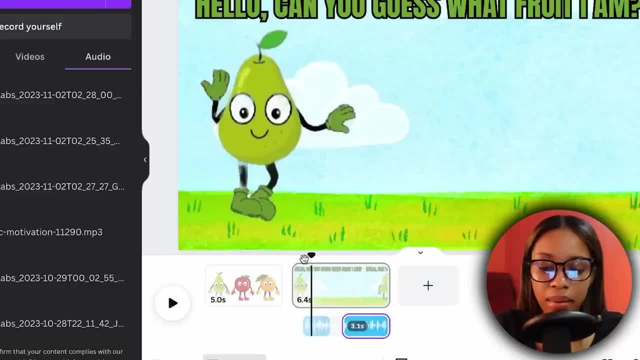 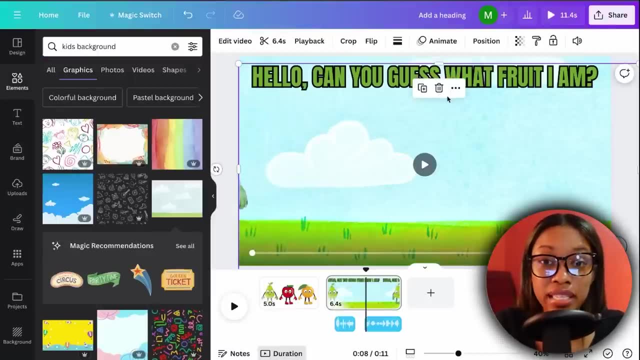 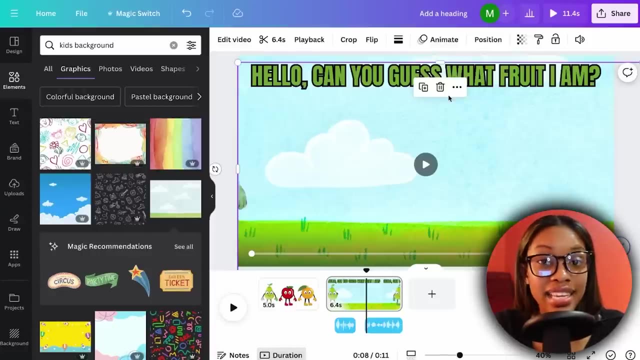 to click split audio. so now let's separate this, and now we can see what this looks like so far. and that's pretty much your first scene done now in order to generate your second scene. it's literally following quite the same process. it's actually even easier. in order to do it, what you want to do is click onto. 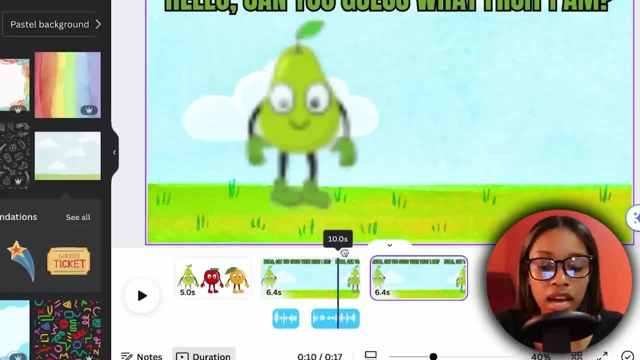 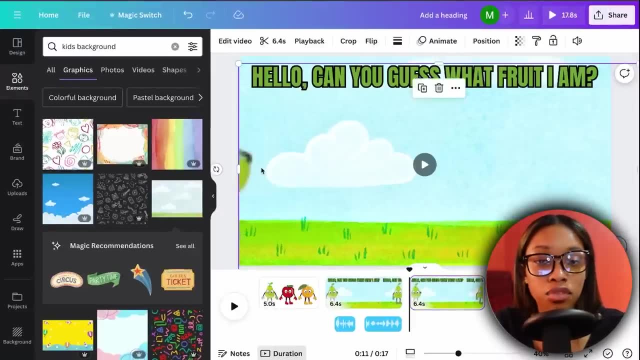 these three dots and then click duplicate page. now you have the page for your second scene already, mostly done from here. what you want to do is click onto the pair because you don't need the same movement. click onto your character and then delete this movement if you no longer need it. 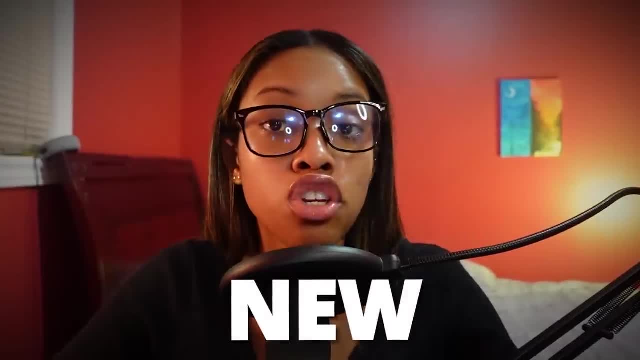 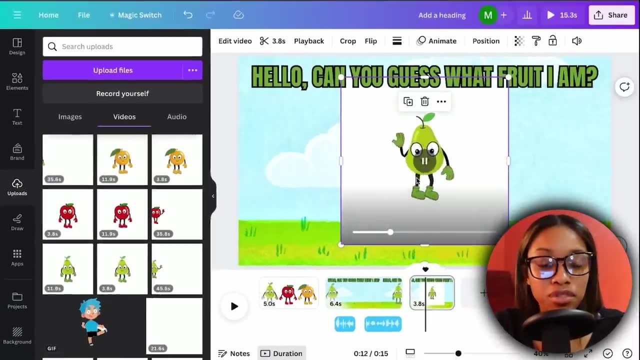 now he's no longer here, then i'm going to now add in the new movement for my second scene. so i'm going to go on to uploads, go to videos and then click the second movement that i needed for my video. now that it's added in, i need to follow the similar process to remove. 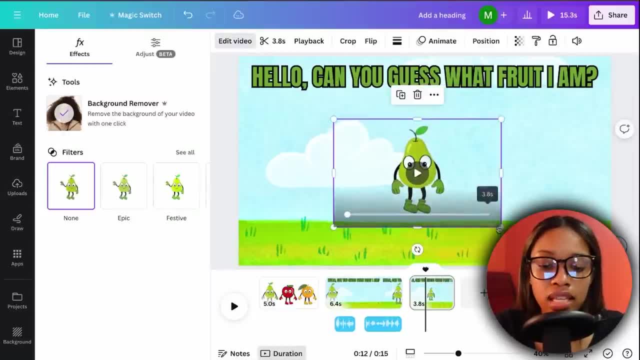 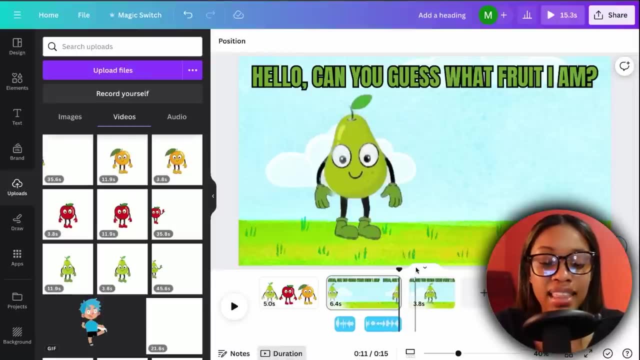 the background. now, once the background is removed, i need to now adjust the sizing and the positioning of the pair so that it's in the same spot that it was in at the ending of the previous animation. so, as you can see, now it's in the same positioning. so what i need to do now is change the text to: 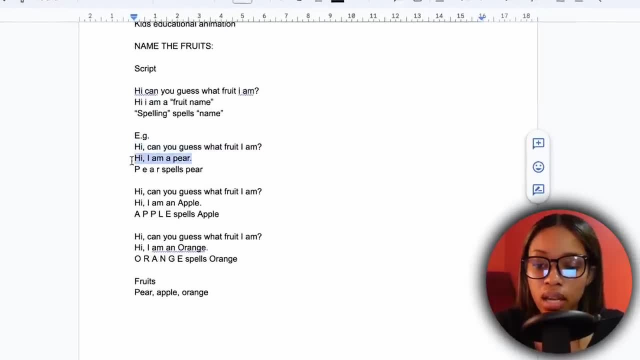 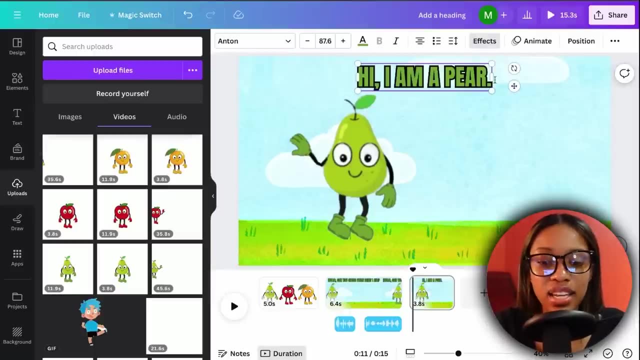 what the second scene says. i'm simply going to go back to my script, copy what it's saying. come back over to canva, double click on the text that's right here, delete it and then paste in the new one, and, as you can see, it's already nicely done and formatted for us. so then, what i need to do now? 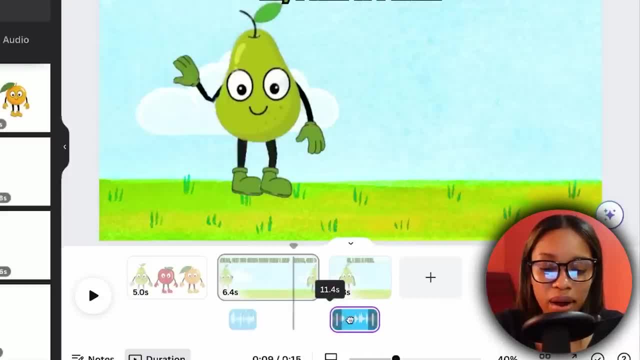 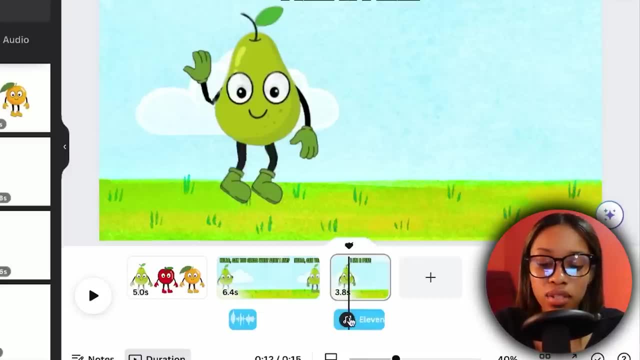 is: take my audio, drag it down to where i want it to start, and then, once you have your audio in, you want to do the same thing. you want to listen to it, and then you want to go ahead to split it where that part ends. so now you have two separated audios, and then that's how easy it is. you'd go. 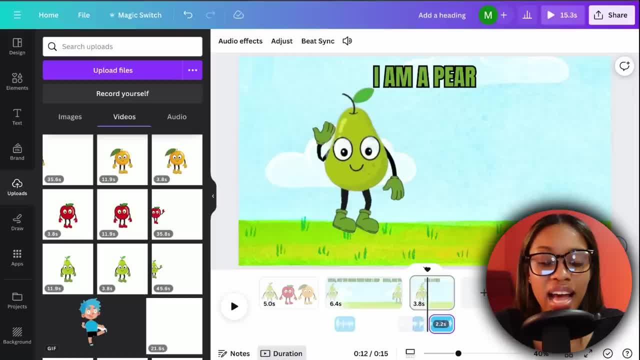 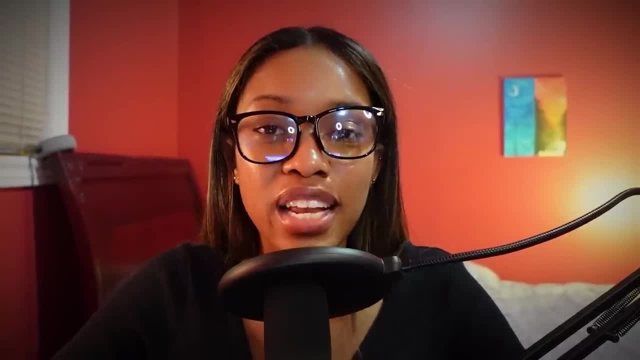 ahead and continue doing the same process for all of your different scenes and for each of your different characters, and set it up in such a way where it's engaging, where it's following through, until you've done your entire video. now, as you can see, i've added in all my different characters. 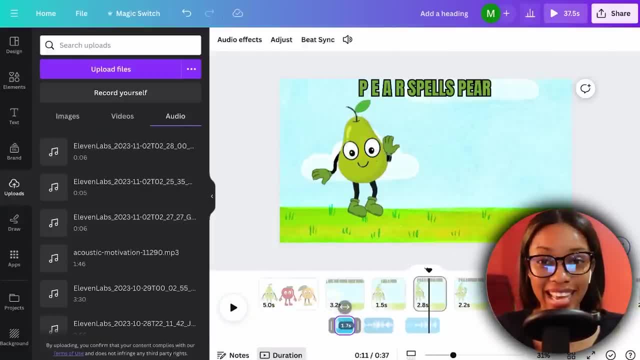 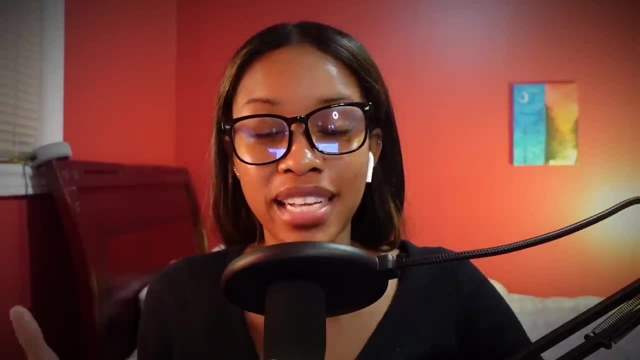 and all my different texts once you're done. that you're not done yet, because the last thing you need to do to truly make this a great video is to add in some background music. you now, in order to find some good background music, we're going to be using the site that I like to. 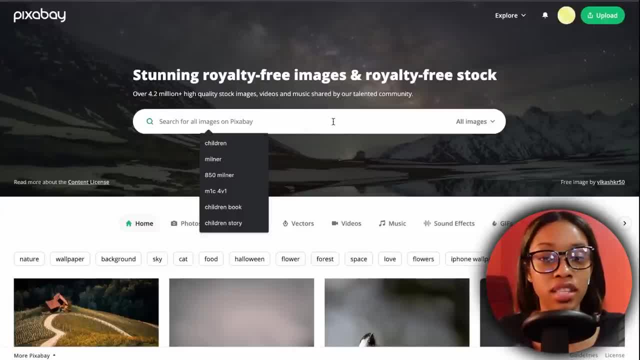 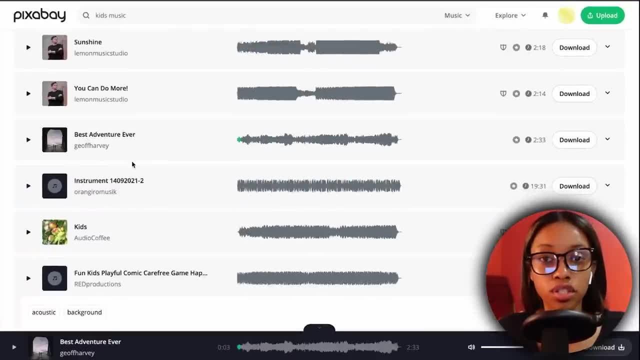 use, called pixabay. once on pixabay, all you need to do is search for the type of music you want and then, over here, be sure you select music and then, as you can see, it's giving me options. so what you want to do is scroll through this, find one that you like, and once you find one that you, 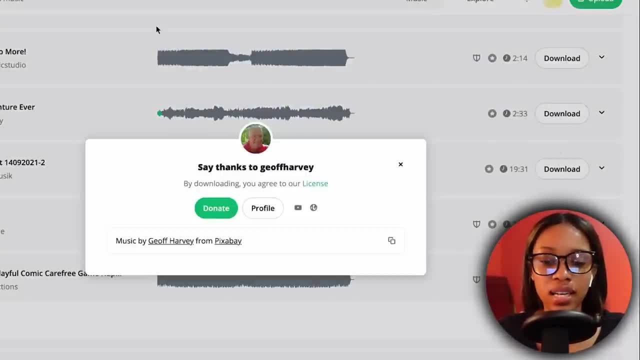 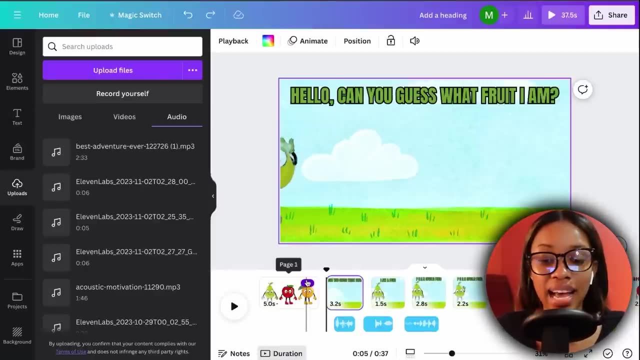 like. in order to download it. all you need to do is click download. once you've done that, you're going to head on back over to canva and upload that music that you just downloaded and now, once it's been added in and showing that our playhead is at the start of our video, you can simply click. 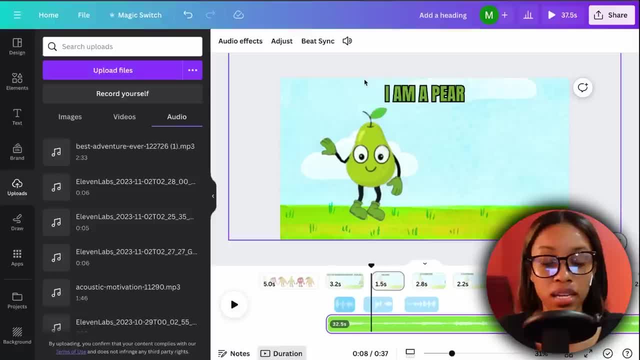 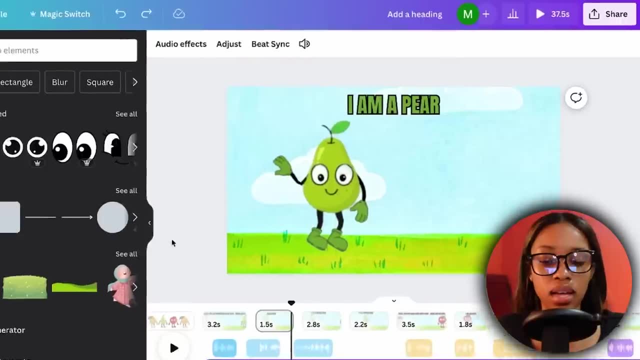 onto it. once your audio is added in, you need to adjust the volume because you don't want it to be too loud. so you'll click onto your audio and then you click this and then you adjust the audio of it and then, once you've done this, you can edit your video even further. you could edit your audio. 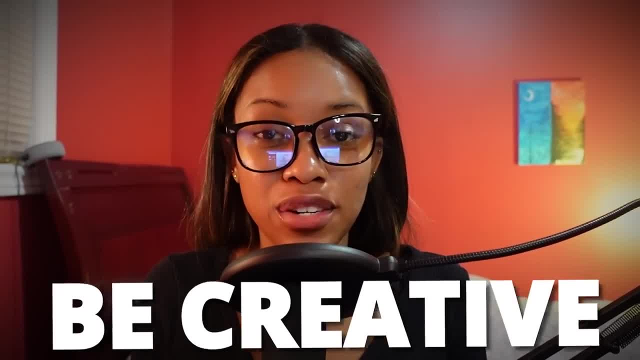 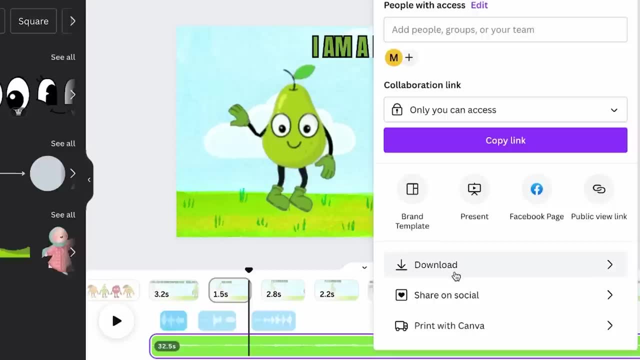 add in sound effects. you could do anything else you want. be as creative as you wish, but once you're done, you need to download your video. in order to download it, so you want to click where it says share, share. you're going to click download and then you're going to leave mp4 and then all you're going to. 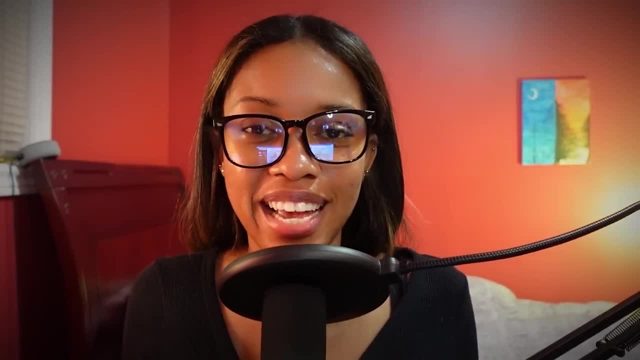 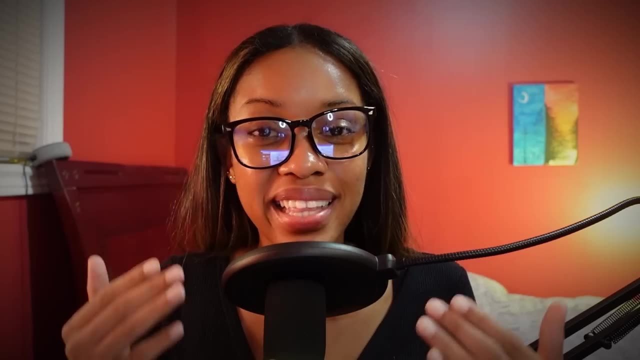 do from here is click download and then you can go ahead and post it to your youtube channel. great job again. so now i know you're probably thinking: thank you for the great tutorial, monique, but like what does this look like? well, let's see what it looks like. hello, can you guess what fruit? 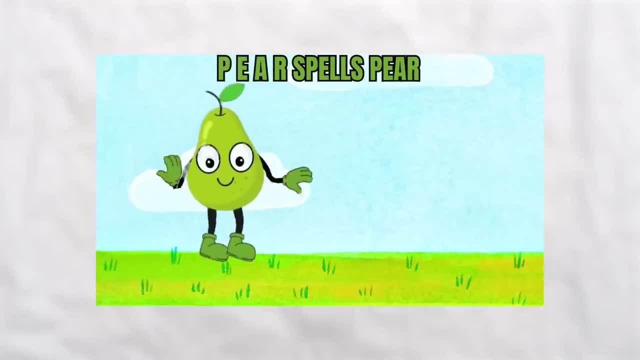 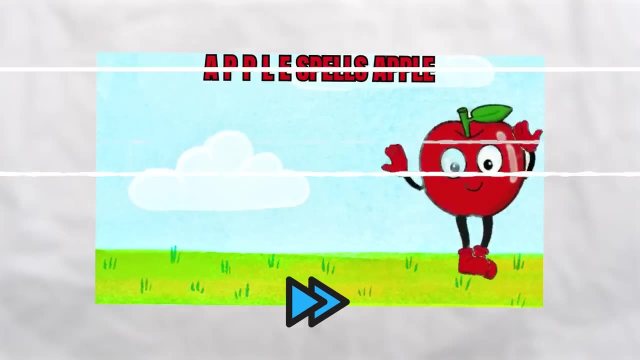 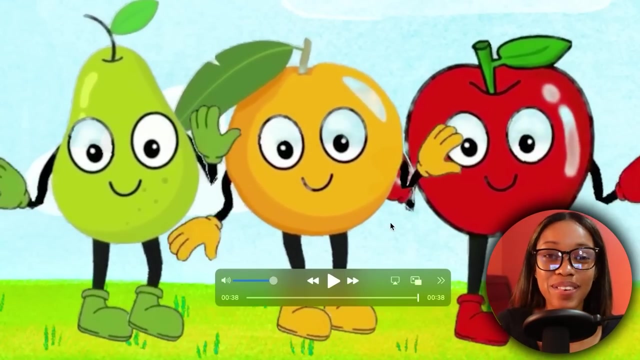 i am. i am a pear. p-e-a-r spells pear. the way they all just did their cute little dance together, that was amazing. now, like i said, remember very well. see there. it may not be the perfect, but with a lot more editing and a lot more. 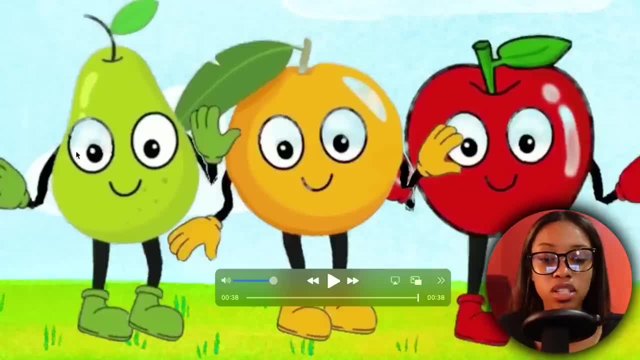 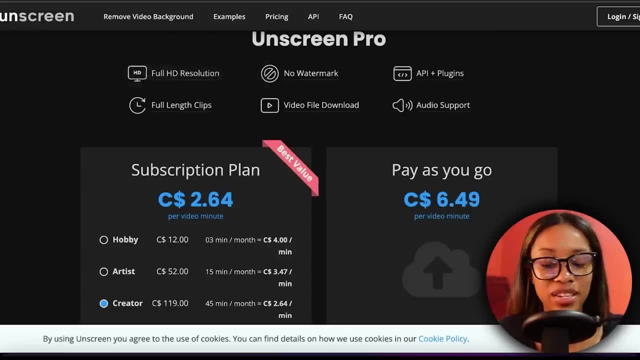 work. you can't get it to use better. and remember what i said: just try your best not to use the color white. if you want, you can completely do the same process, but use unscreen instead so that you could have your perfect character. and remember: if you want to grow fast, you need to be unique. say it with me, everybody.